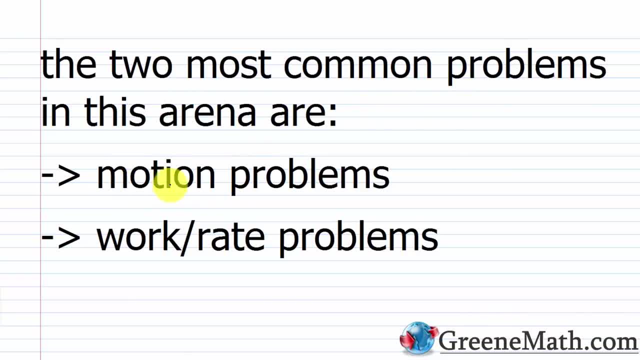 two most common problems in this arena are going to be motion word problems which we saw back at the beginning of Algebra 1. You might use your distance formula there. Distance is equal to rate of speed times, the amount of time traveled. And then something that's new to us is going to be: 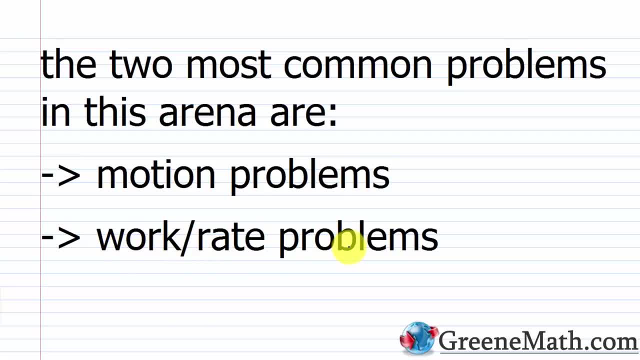 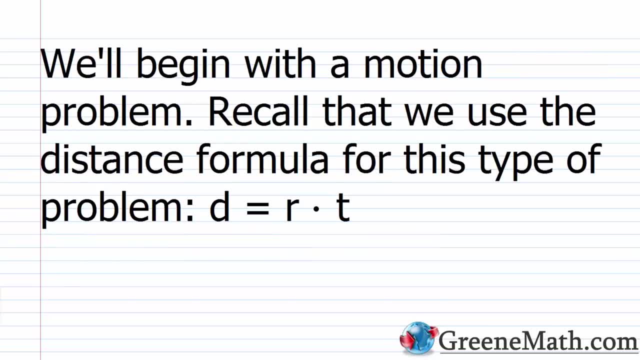 these work rate problems, or some people say rate of work problems. So these are really, really easy to solve. We're going to get to them at the very end of the lesson, All right, so we're going to begin today with a motion word problem. So I want you to recall that we use the 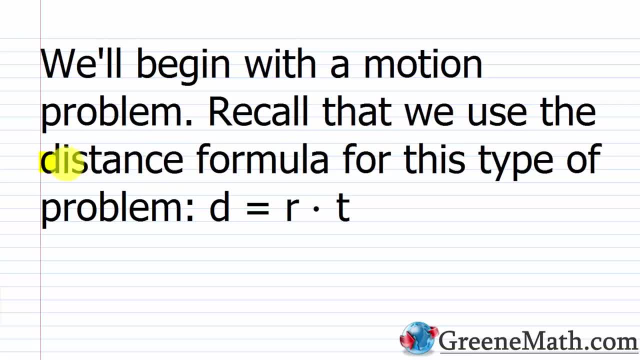 distance formula. Let me just highlight that real quick. The distance formula for this type of problem. So we have: d is equal to r times c, T. Remember this: D stands for distance, the R stands for rate of speed and T stands for time. 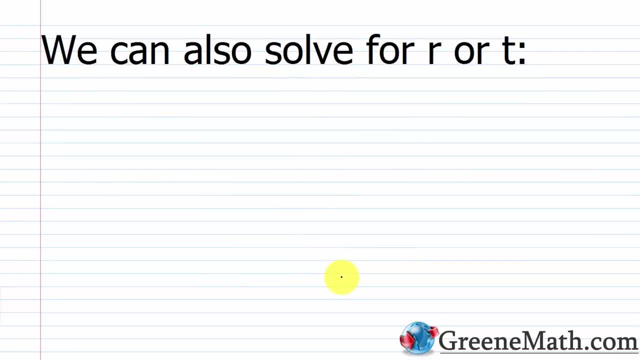 traveled. So something that's going to be new for us here is that we're going to manipulate the distance formula and we're going to be solving it for R or T. So, for example, if I have distance is equal to rate- times, time- and I want to solve this for the rate- Let me highlight that- How would I? 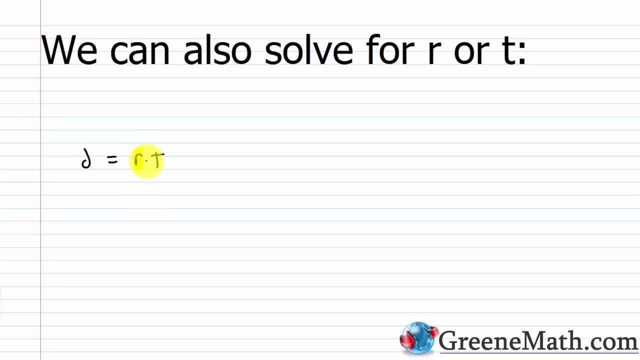 go about doing that. Well, all we're going to do is realize that if T is multiplying R to get R by itself, I just divide both sides of the equation by T And what's going to happen is the T is going to cancel here and here, and on the right side of the equation I'm just left with R. It's isolated. 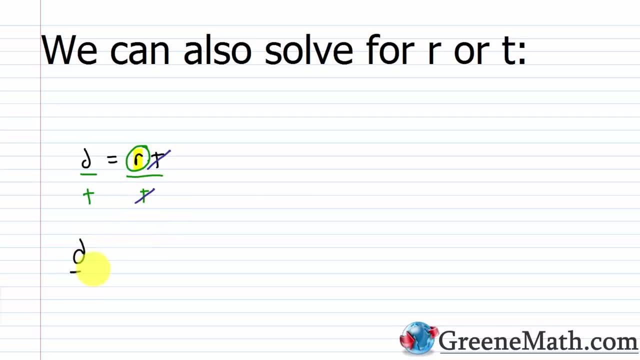 and so what I have is I have a distance of time traveled, So I'm going to do that I'm going to have. distance over time is equal to rate. Now let's check that real quick and make sure that that makes sense. We know from the traditional distance formula that if I am going, let's say 40. 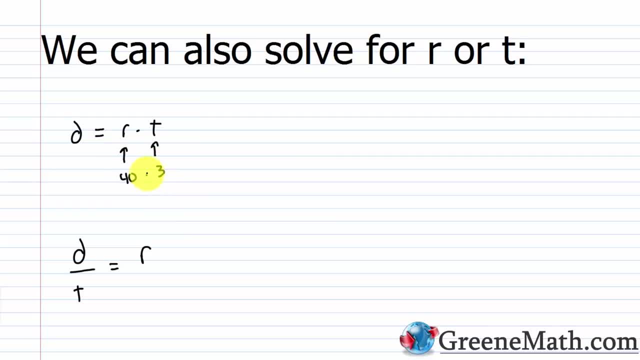 miles per hour and I do this for three hours. 40 times 3 is 120.. I've traveled 120 miles. Okay, so that makes sense. If I plug in the same numbers here, is that going to work? So if I plugged in? 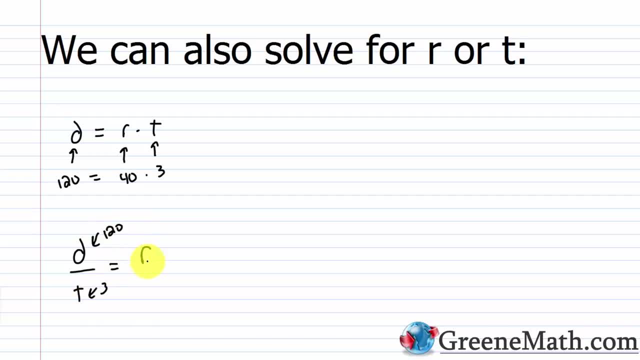 120. here I'm going to have 120 miles per hour. So if I plug in the same numbers here, is that going to work? So if I plug in the same numbers here and I plugged in a 3 here, would I get 40. 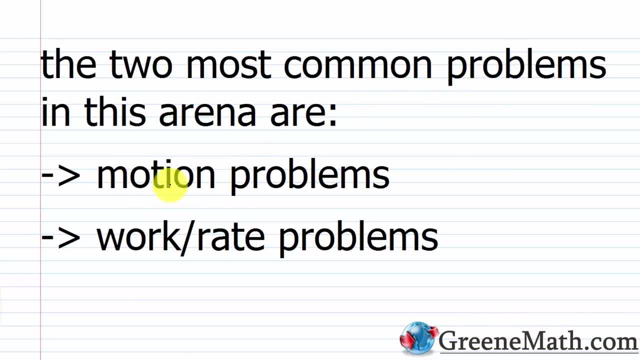 two most common problems in this arena are going to be motion word problems which we saw back at the beginning of Algebra 1. You might use your distance formula there. Distance is equal to rate of speed times, the amount of time traveled. And then something that's new to us is going to be: 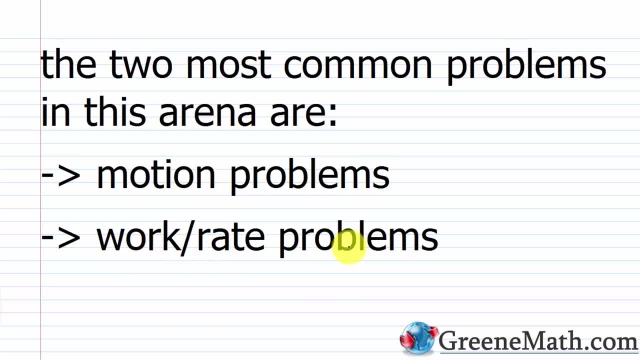 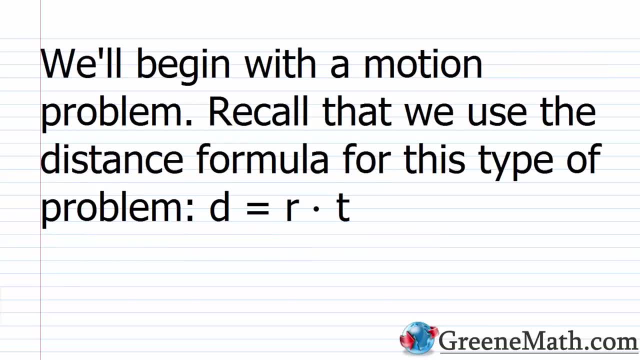 these work rate problems, or some people say rate of work problems. So these are really, really easy to solve. We're going to get to them at the very end of the lesson, All right? so we're going to begin today with a motion word problem. So I want you to recall that. 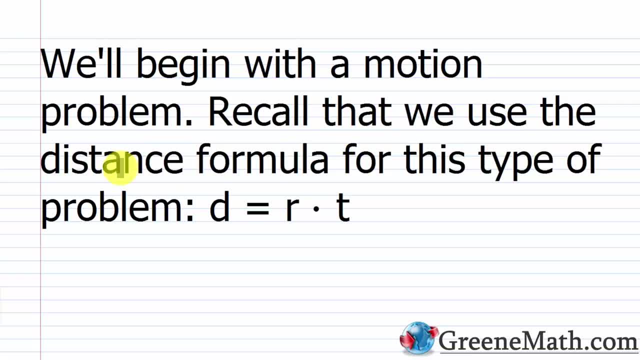 we use the distance formula. Let me just highlight that real quick: The distance formula for this type of problem. So we have: d is equal to r times t And we're going to use the distance formula, T. Remember this: D stands for distance, the R stands for rate of speed and T stands for time. 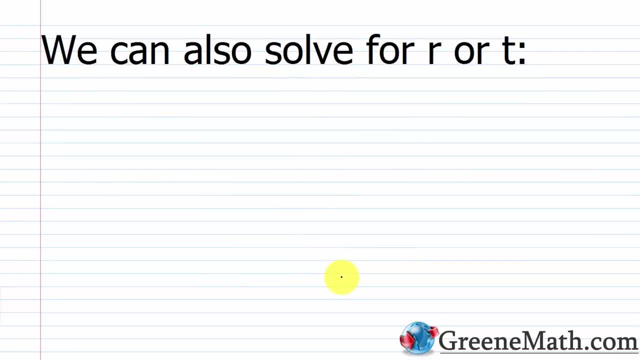 traveled. So something that's going to be new for us here is that we're going to manipulate the distance formula and we're going to be solving it for R or T. So, for example, if I have distance is equal to rate- times, time- and I want to solve this for the rate- Let me highlight that- How would I? 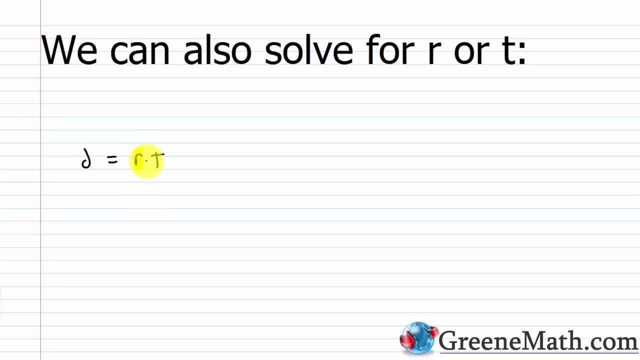 go about doing that. Well, all we're going to do is realize that if T is multiplying R to get R by itself, I just divide both sides of the equation by T And what's going to happen is the T is going to cancel here and here, and on the right side of the equation I'm just left with R. It's isolated. 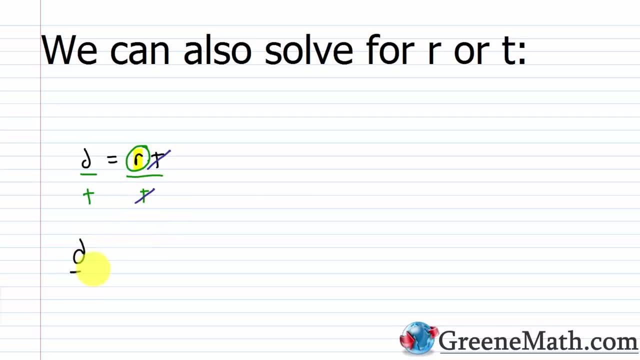 and so what I have is I have a distance of time traveled, So I'm going to do that I'm going to have. distance over time is equal to rate. Now let's check that real quick and make sure that that makes sense. We know from the traditional distance formula that if I am going, let's say 40. 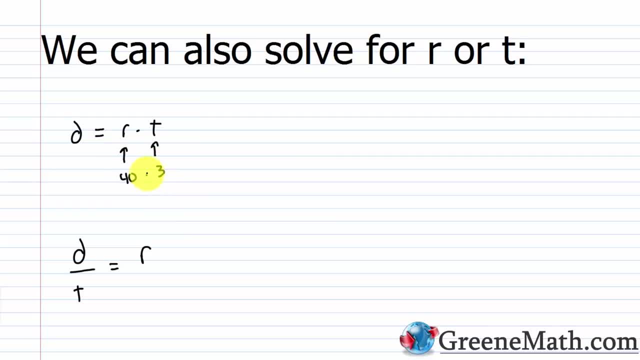 miles per hour and I do this for three hours. 40 times 3 is 120.. I've traveled 120 miles. Okay, so that makes sense. If I plug in the same numbers here, is that going to work? So if I plugged in? 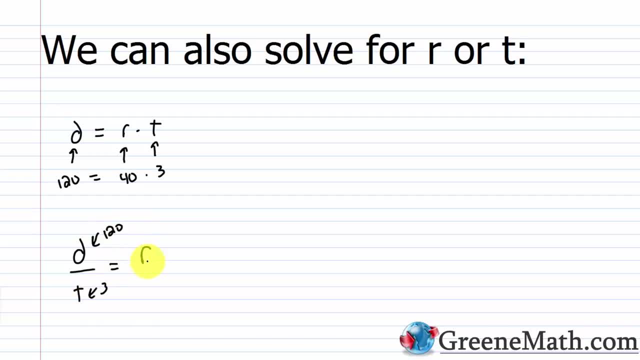 120. here I'm going to have 120 miles per hour. So if I plug in the same numbers here, is that going to work? So if I plug in the same numbers here and I plugged in a 3 here, would I get 40. 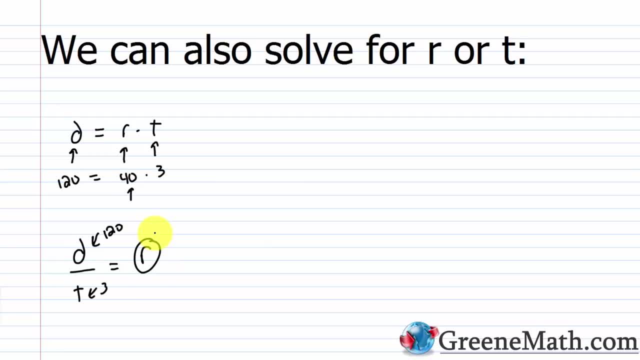 here. Well, yes, I would. 120 divided by 3 is in fact 40. Right, so we're good to go there. Now the other thing we might have to solve for is time. So if I have distance is equal to rate times time, I'm going to use the same logic to solve for time. I want to isolate this guy, so 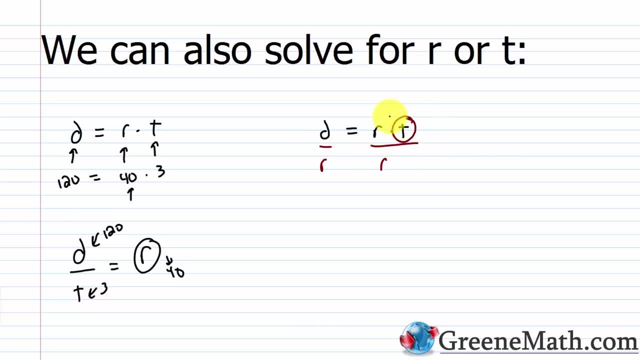 I'm going to divide both sides of the equation by R so I can isolate the T. Let's cancel this and I'm going to be left with. time is equal to distance over rate And again you can say: okay, using this example, if I plugged in 120 here and I plugged in a 40 there, 120 divided by 40 is in. 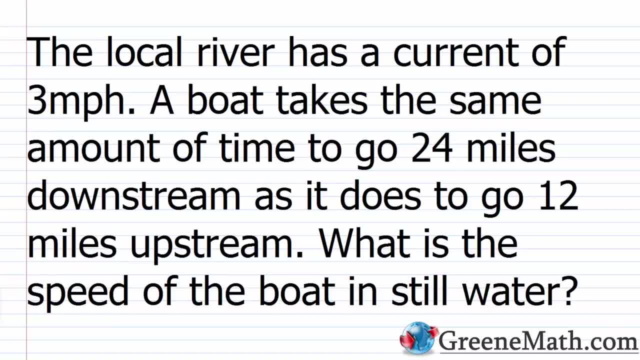 fact 3. So we're good to go. Alright, so let's go ahead and take a look at the first problem. So the local river has a current of 3 miles per hour. A boat takes the same amount of time to go 24 miles. 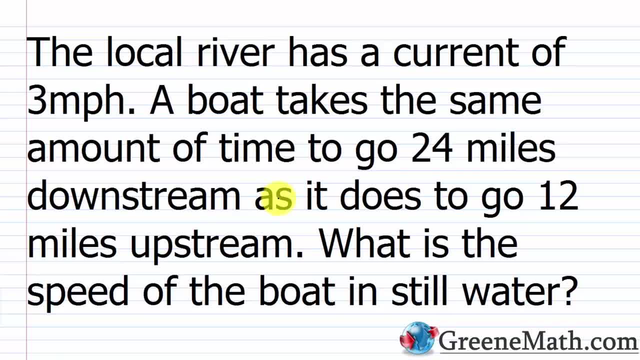 upstream. okay, that's going with the current. in case you don't know that, as it does to go 12 miles upstream. Upstream is against the current. What is the speed of the boat in still water? So it might seem like this is a difficult problem, but it's really not. Let's go ahead and make a little table. 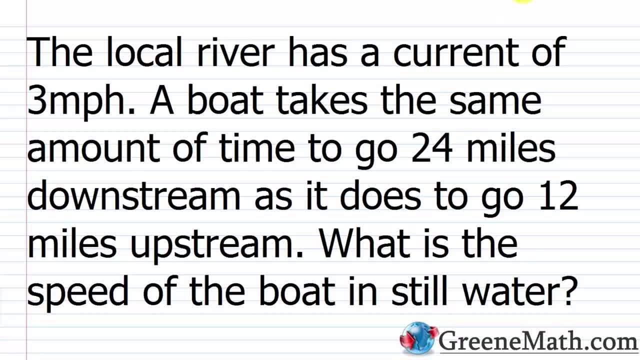 to kind of organize our information. The two things we're going to think about is the scenario where we're going downstream- again, that's with the current- and the scenario where we're going to go upstream, and that's against the current. Let's scroll down here real quick, So we'll kind of 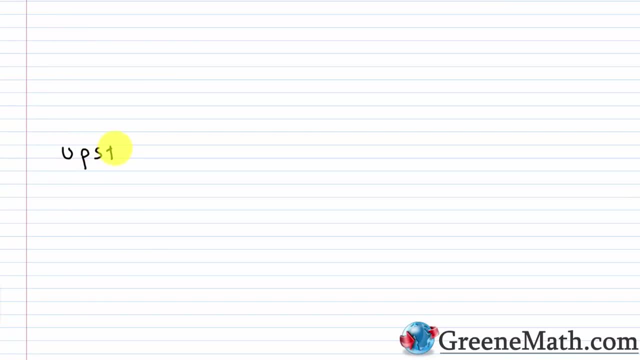 think about: okay, we have upstream and we have downstream, Okay. so let me just draw a little line here. Now, the components of the distance formula. let's think about those. So we have distance. so I'm just going to abbreviate with a d We have 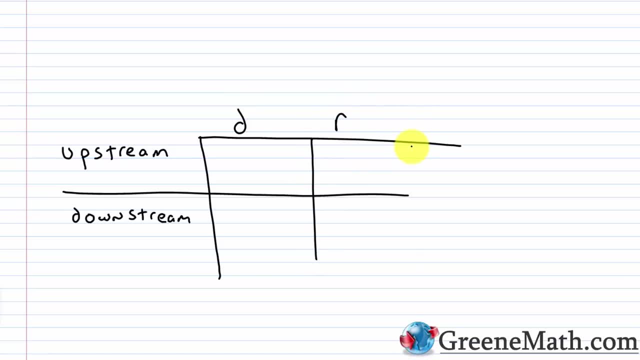 the rate of speed, which I'm going to use an r for, and then we have the time. So what I want to do here is just fill in this table and get the information that I'm going to need to create an equation that's going to allow me to solve and figure out an answer for this problem. Let's scroll. 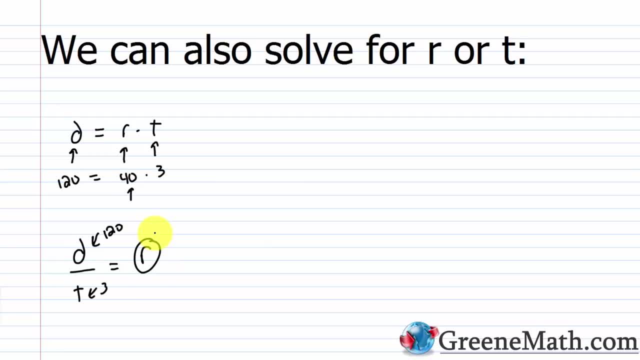 here. Well, yes, I would. 120 divided by 3 is in fact 40. Right, so we're good to go there. Now the other thing we might have to solve for is time. So if I have distance is equal to rate times time, I'm going to use the same logic to solve for time. I want to isolate this guy, so 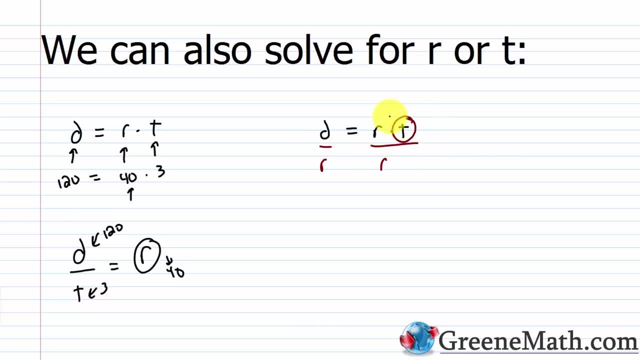 I'm going to divide both sides of the equation by R so I can isolate the T. Let's cancel this and I'm going to be left with. time is equal to distance over rate And again you can say: okay, using this example, if I plugged in 120 here and I plugged in a 40 there, 120 divided by 40 is in. 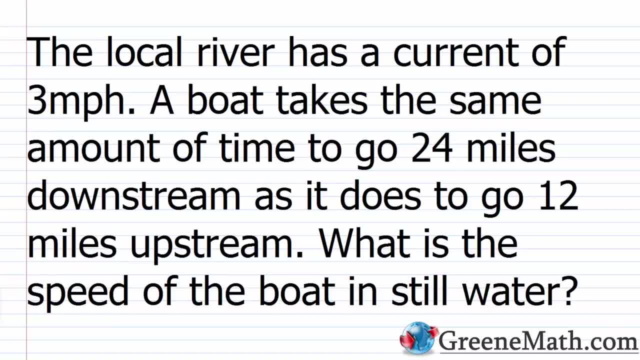 fact 3. So we're good to go. Alright, so let's go ahead and take a look at the first problem. So the local river has a current of 3 miles per hour. A boat takes the same amount of time to go 24 miles. 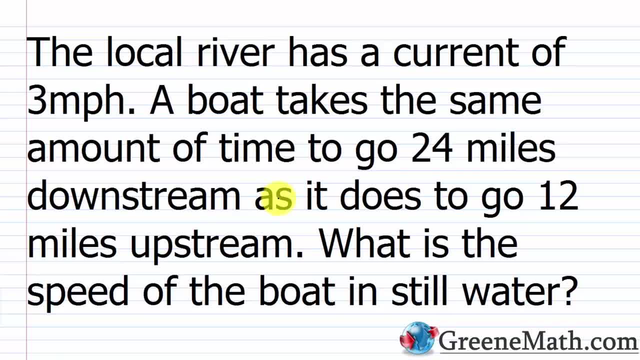 upstream. okay, that's going with the current. in case you don't know that, as it does to go 12 miles upstream. Upstream is against the current. What is the speed of the boat in still water? So it might seem like this is a difficult problem, but it's really not. Let's go ahead and make a little table. 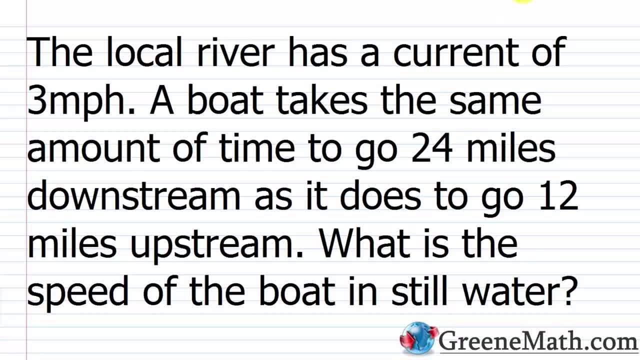 to kind of organize our information. The two things we're going to think about is the scenario where we're going downstream- again, that's with the current- and the scenario where we're going to go upstream, and that's against the current. Let's scroll down here real quick, So we'll kind of 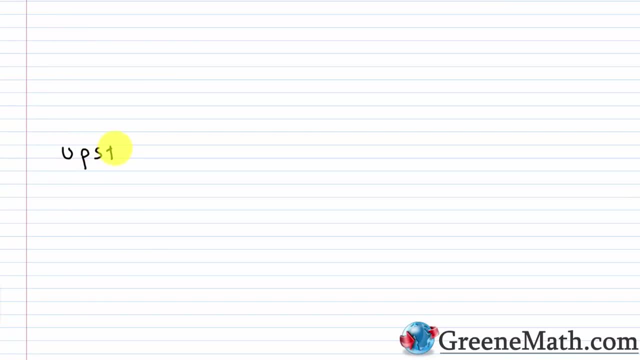 think about: okay, we have upstream and we have downstream, Okay. so let me just draw a little line here. Now, the components of the distance formula. let's think about those. So we have distance. so I'm just going to abbreviate with a d We have 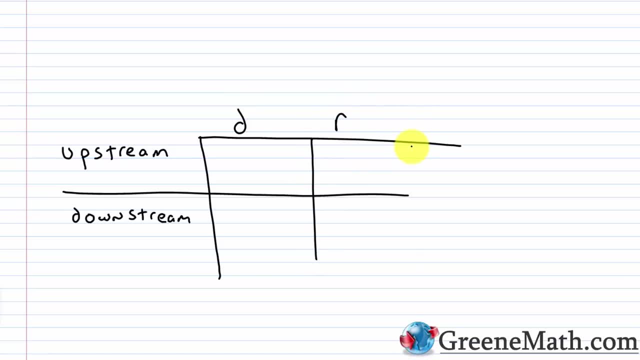 the rate of speed, which I'm going to use an r for, and then we have the time. So what I want to do here is just fill in this table and get the information that I'm going to need to create an equation that's going to allow me to solve and figure out an answer for this problem. Let's scroll. 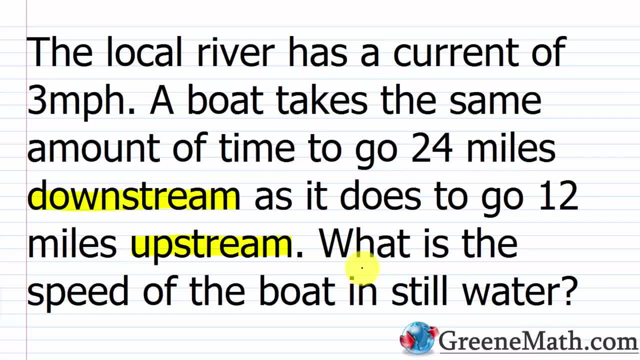 back up to the top real quick. Alright. so it tells us in the problem that the boat is going 24 miles upstream. So what we're going to do here is we're going to put the time as it does to go 12 miles upstream. So for the distance, I'm going to put 24 miles under downstream and 12 miles under upstream. 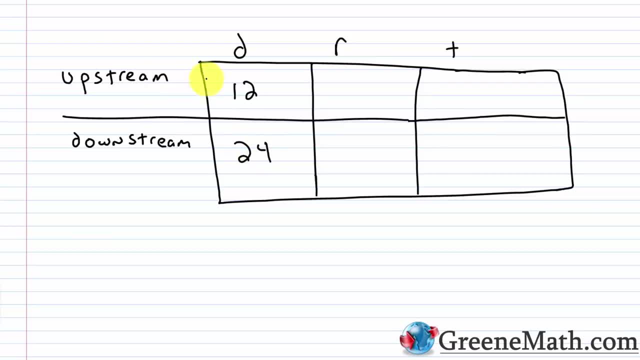 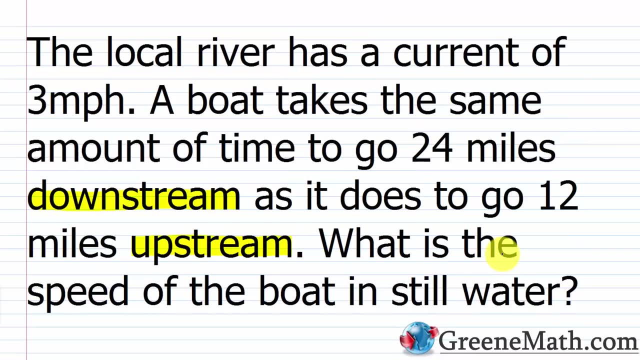 Okay, so I'm going to write 12 here and 24 here Again. the distance when I'm going upstream is 12 miles. the distance when I'm going downstream is 24 miles. Now let's think about the rate. So when we think about the rate of speed, again, this is how fast we're traveling, the only information we're. 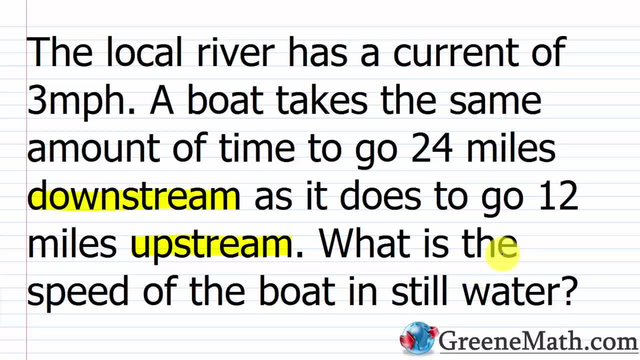 going to get is the current of 3 miles per hour. It doesn't give us any other information. Now, what you're supposed to know here is that if you're going upstream, you are fighting the current right. So, whatever the amount of speed you're going in miles per hour like if you're going 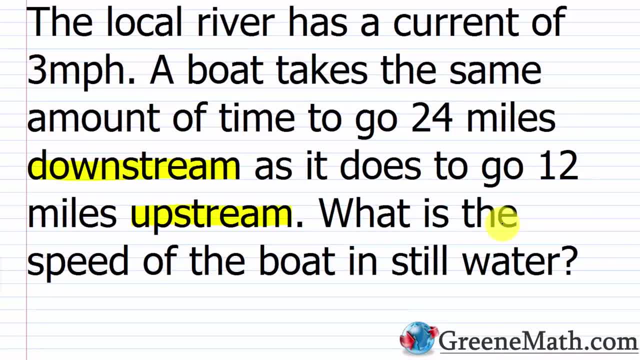 in still water. you've got to subtract 3 away from that because you're fighting the current. So if I let a variable like x- let's say let x equal the speed of the boat in still water- Well, what happened is the speed when I'm going upstream would be x. 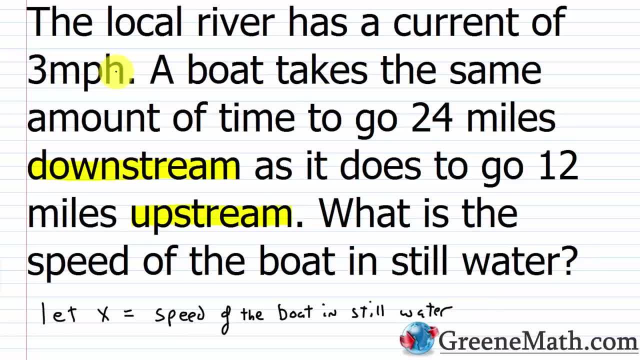 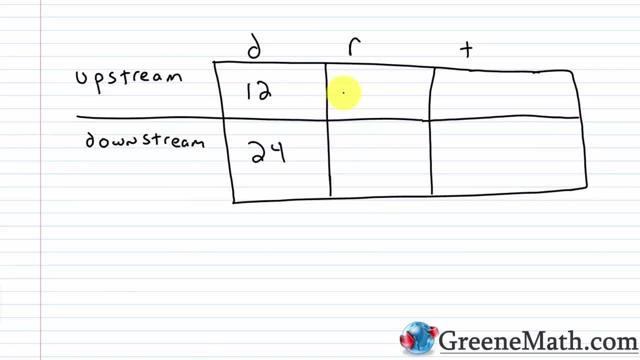 the speed of the boat in still water minus 3, because that's the speed of the current and that's what I'm fighting. So let's scroll down and put that So again, for the upstream speed it's going to be x: the speed of the boat in still water minus 3, the speed of 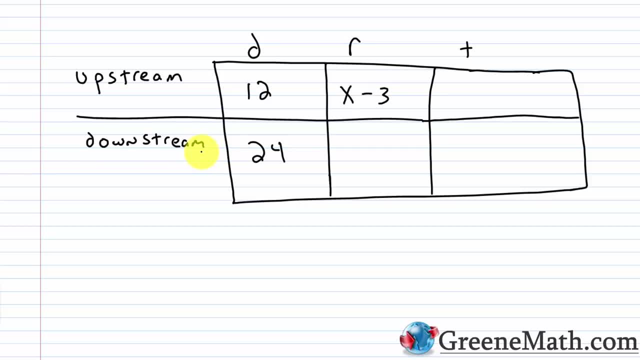 the current, And then for the downstream speed it's just as easy, right? We think about. the speed of the boat in still water is x, And then now, if I'm going downstream, that means I'm going with the current. So the current is pushing on my boat. It's making me go faster by 3 miles an hour, So I 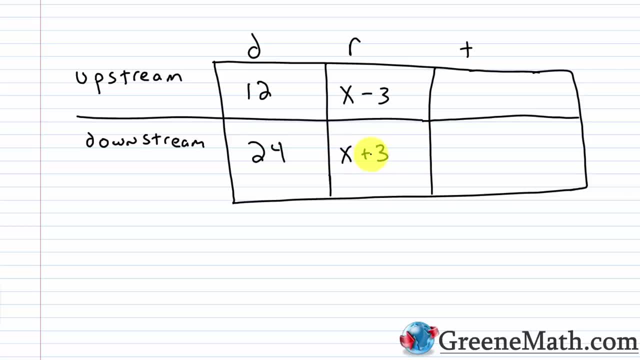 would add 3 to that x. So x plus 3 is the speed of the boat going downstream, x minus 3 is the speed of the boat going upstream. Now, how do I go about getting a time? Well, reading back through the problem, the only thing it really. 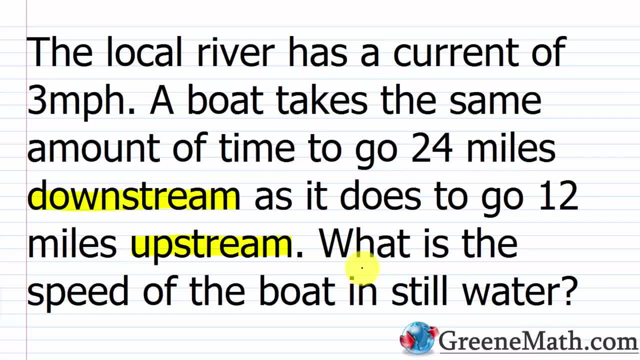 back up to the top real quick. Alright. so it tells us in the problem that the boat is going 24 miles upstream. So what we're going to do here is we're going to put the time as it does to go 12 miles upstream. So for the distance, I'm going to put 24 miles under downstream and 12 miles under upstream. 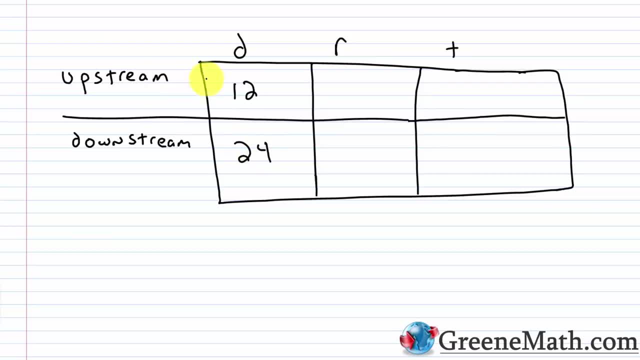 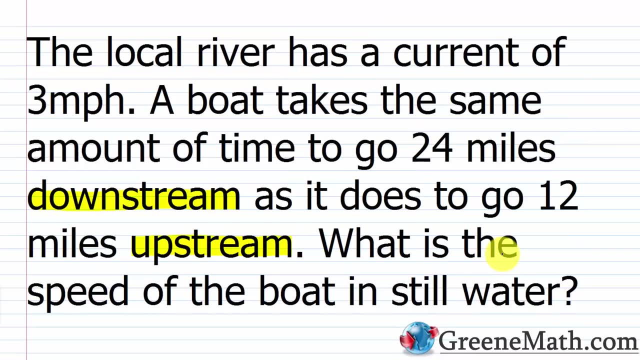 Okay, so I'm going to write 12 here and 24 here Again. the distance when I'm going upstream is 12 miles. the distance when I'm going downstream is 24 miles. Now let's think about the rate. So when we think about the rate of speed, again, this is how fast we're traveling, the only information we're. 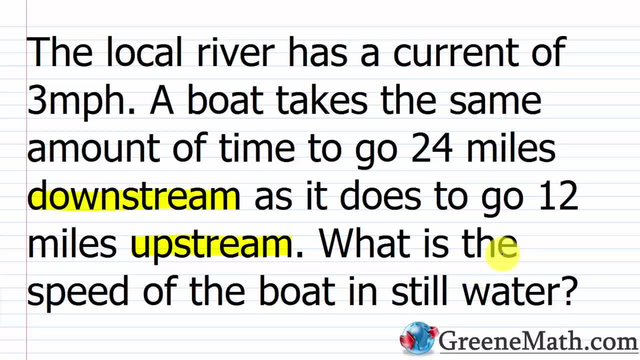 going to get is the current of 3 miles per hour. It doesn't give us any other information. Now, what you're supposed to know here is that if you're going upstream, you are fighting the current right. So, whatever the amount of speed you're going in miles per hour like if you're going 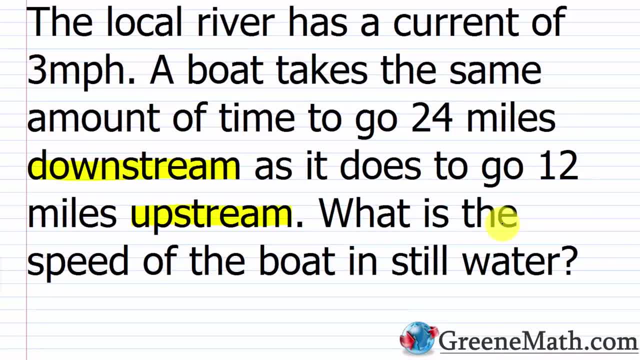 in still water. you've got to subtract 3 away from that because you're fighting the current. So if I let a variable like x- let's say let x equal the speed of the boat in still water- Well, what happened is the speed when I'm going upstream would be x. 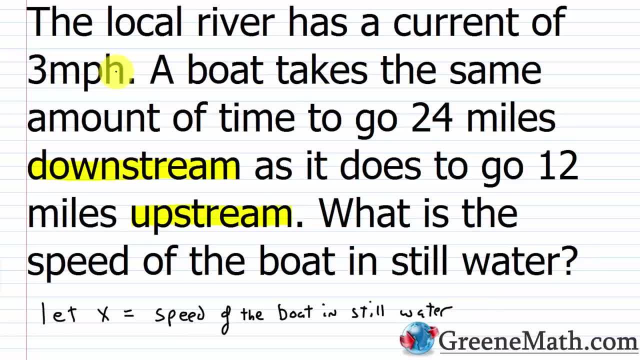 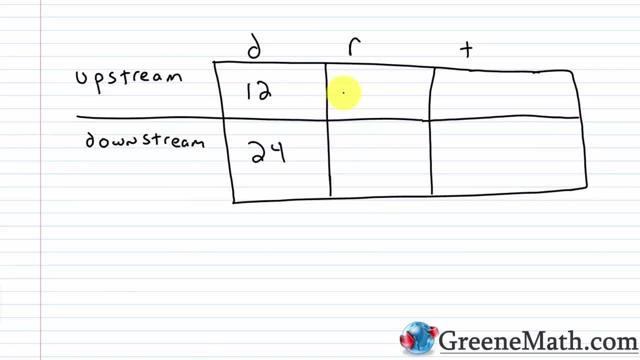 the speed of the boat in still water minus 3, because that's the speed of the current and that's what I'm fighting. So let's scroll down and put that So again, for the upstream speed it's going to be x: the speed of the boat in still water minus 3, the speed of 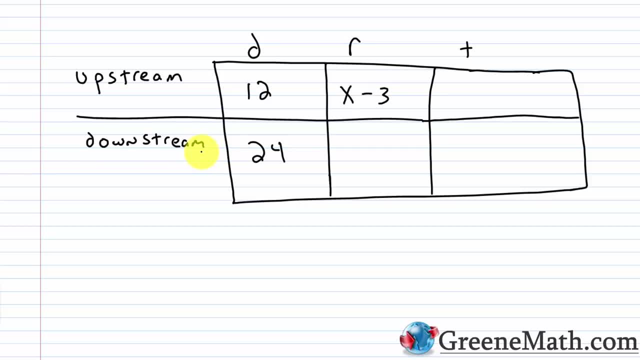 the current, And then for the downstream speed it's just as easy, right? We think about. the speed of the boat in still water is x, And then now, if I'm going downstream, that means I'm going with the current. So the current is pushing on my boat. It's making me go faster by 3 miles an hour, So I 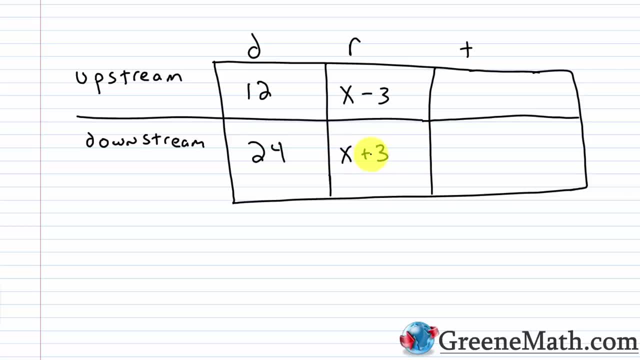 would add 3 to that x. So x plus 3 is the speed of the boat going downstream, x minus 3 is the speed of the boat going upstream. Now, how do I go about getting a time? Well, reading back through the problem, the only thing it really. 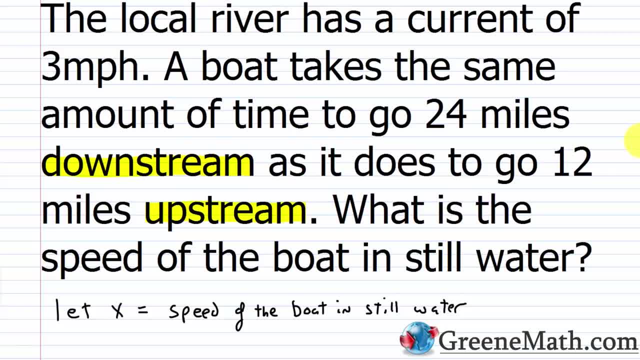 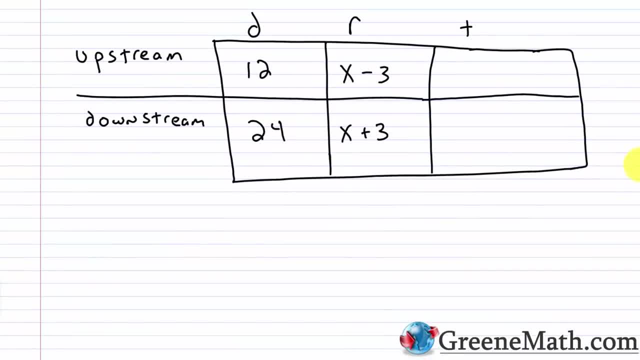 says about the time is that it takes the same amount of time to go 24 miles downstream as it does to go 12 miles upstream. So what I can do here, as we talked about a little while ago, is I can get a time for each one and then I can set those times equal to each other. 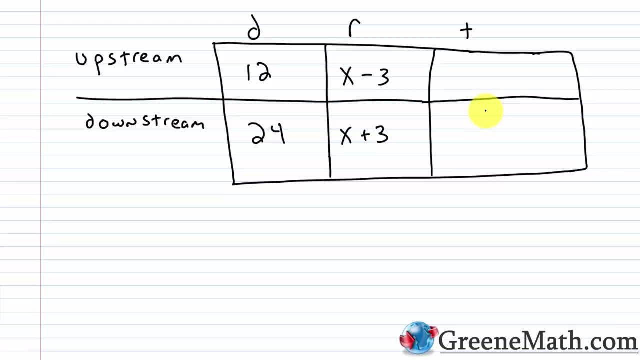 So let's take that one step at a time To get a time. remember the d equals r times t can be solved for t. So if I divide both sides of the equation by r to isolate t, as we did earlier, this cancels with this and I've got t by itself. So time is equal to distance over. 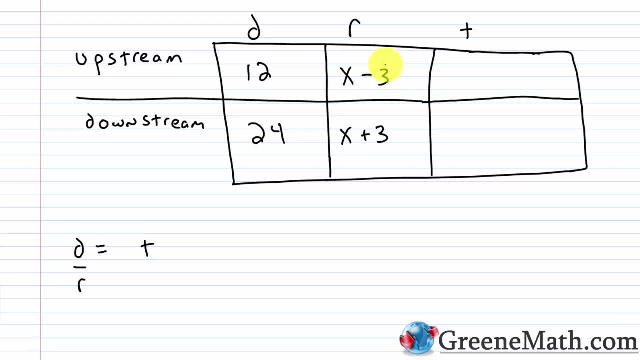 rate. I have a distance here. I have a rate here, So I'm going to have a time. The distance in this case is 12.. The rate in this case is x minus 3.. So my time for going upstream is 12.. 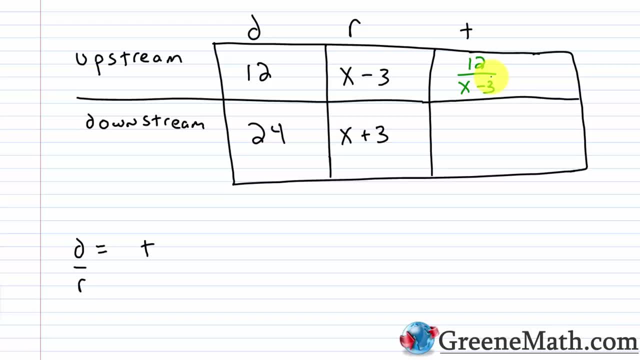 Over x minus 3.. Now for downstream. I can do the same exact thing. My time is going to be 24,, which is my distance over x plus 3,, which is my rate. Now that we have all this information figured out, we want to go ahead and set up an equation And, as I told you, when we look at this, 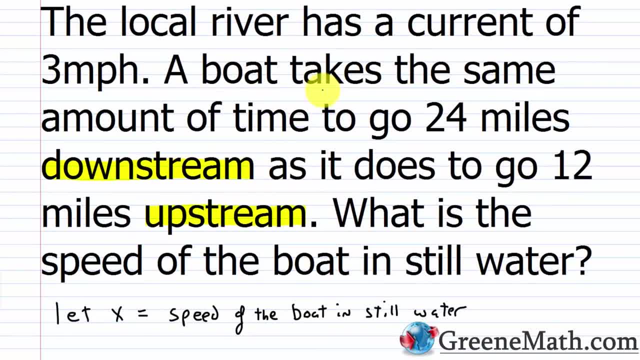 problem. it tells us that a boat takes the same amount of time, the same amount of time, to go 24 miles downstream as it does to go 12 miles downstream. So I'm going to go 24 miles downstream As it does to go 12 miles upstream. So that means I could set the two times equal to each other. 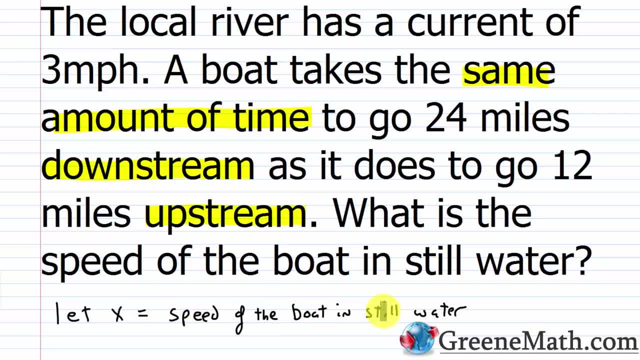 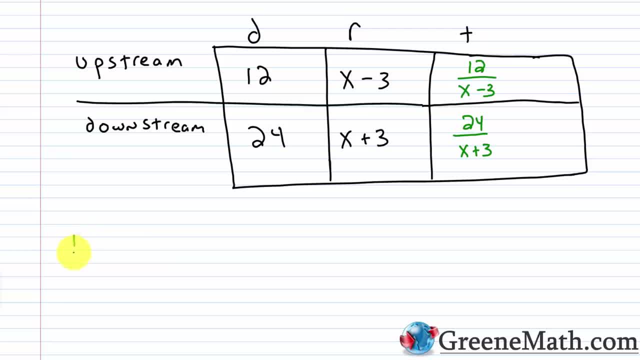 and I could solve for x and I'd figure out what the speed of the boat is in still water. Let me erase this real quick. So I have the time for upstream, which is 12 over x minus 3. And I'm 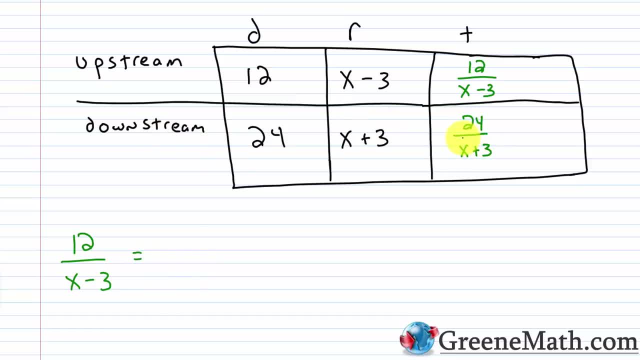 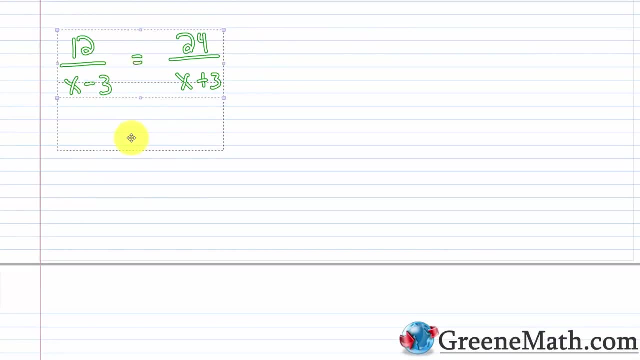 going to set this equal to the time for downstream, which is 24 over x plus 3.. So in the last section we learned how to solve equations of this form. We learned that, and let me kind of scroll this part down. So one way we 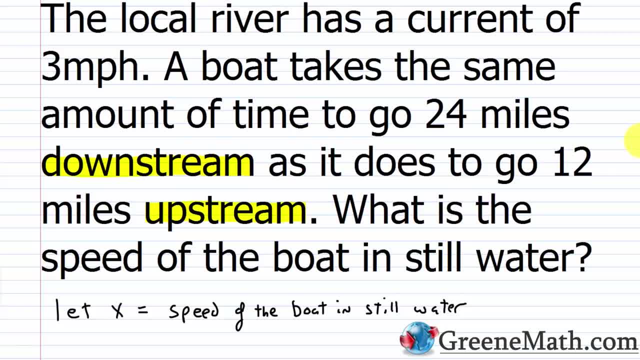 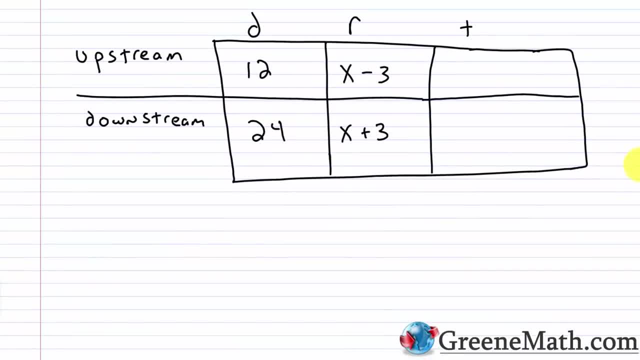 says about the time is that it takes the same amount of time to go 24 miles downstream as it does to go 12 miles upstream. So what I can do here, as we talked about a little while ago, is I can get a time for each one and then I can set those times equal to each other. 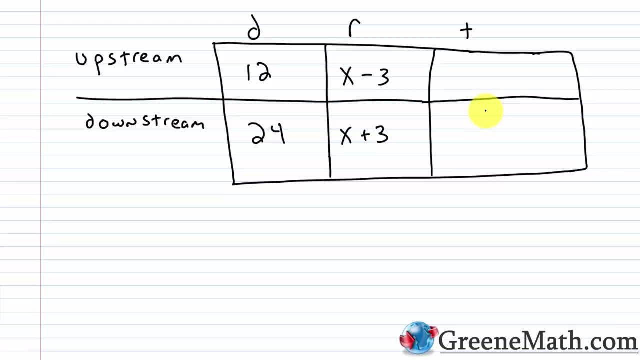 So let's take that one step at a time To get a time. remember the d equals r times t can be solved for t. So if I divide both sides of the equation by r to isolate t, as we did earlier, this cancels with this and I've got t by itself. So time is equal to distance over. 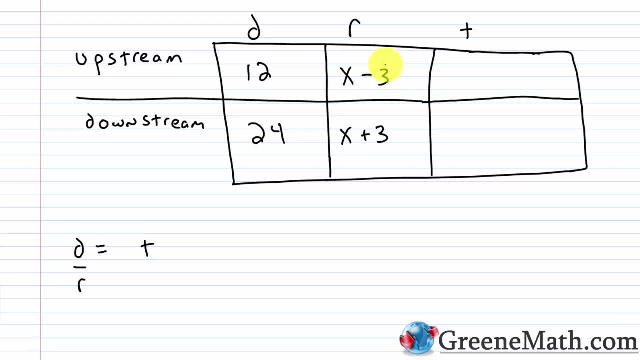 rate. I have a distance here. I have a rate here, So I'm going to have a time. The distance in this case is 12.. The rate in this case is x minus 3.. So my time for going upstream is 12.. 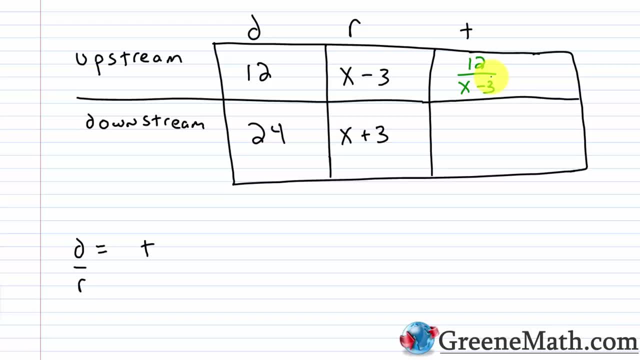 Over x minus 3.. Now for downstream. I can do the same exact thing. My time is going to be 24,, which is my distance over x plus 3,, which is my rate. Now that we have all this information figured out, we want to go ahead and set up an equation And, as I told you, when we look at this, 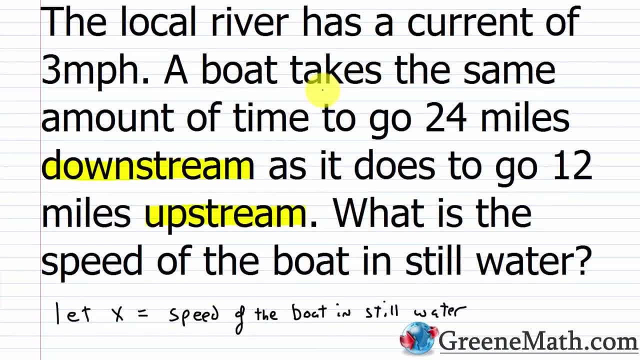 problem. it tells us that a boat takes the same amount of time, the same amount of time, to go 24 miles downstream as it does to go 12 miles downstream. So I'm going to go 24 miles downstream As it does to go 12 miles upstream. So that means I could set the two times equal to each other. 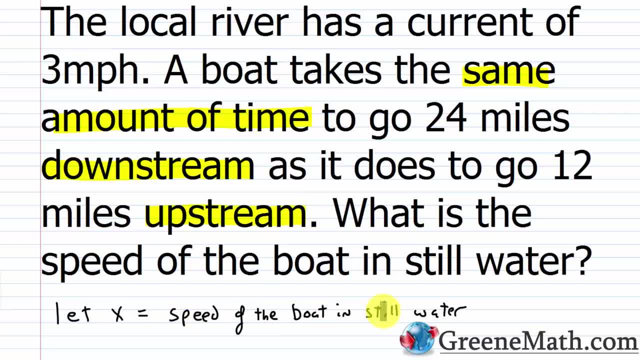 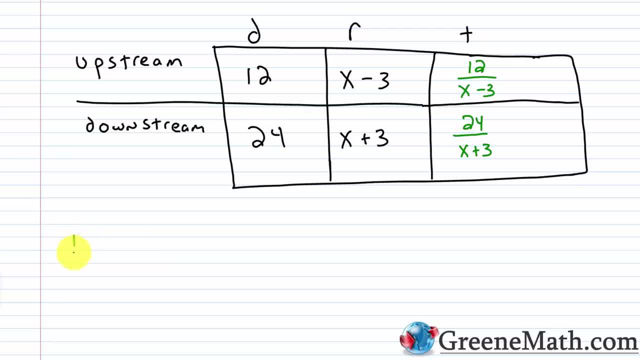 and I could solve for x and figure out what the speed of the boat is in still water. Let me erase this real quick. So I have the time for upstream, which is 12 over x minus 3.. I'm going to set this. 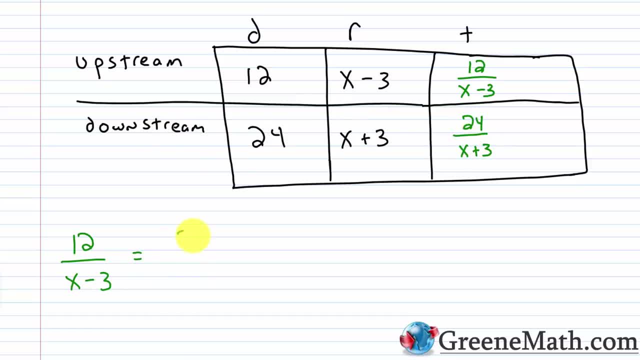 equal to the time for downstream, which is 24 over x plus 3.. So in the last section we learned how to solve a quick equation for downstream. So I'm going to go ahead and do that. So I'm going to go. 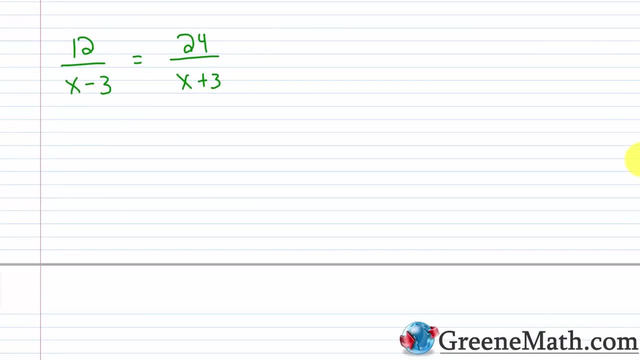 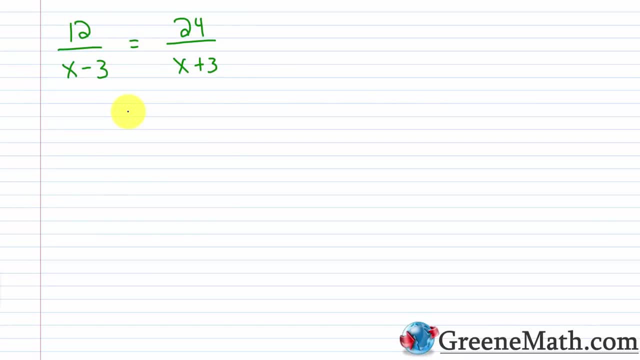 down. So one way we can do this is we can find the LCD and multiply both sides of the equation by the LCD, clear the equation of any denominators and kind of go from there. But if this particular scenario, the easiest thing to do would be to cross-multiply. 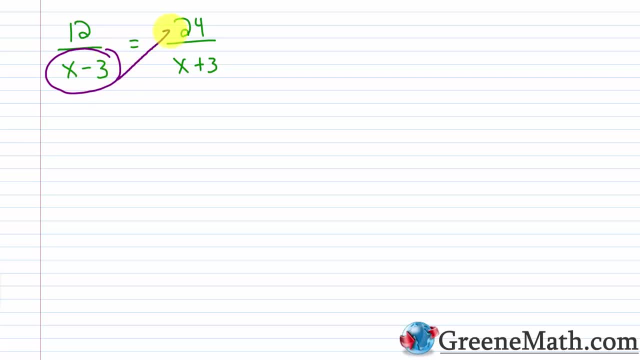 Remember that from proportions, right, I can multiply x ui23.e4 times 24, and I could multiply x plus 3x e3 times 24.. E's all there: x and cinema, x minus 3.. So oftentimes I can have a bunch, but sorry, because normally you'll always need to use that number and half x times 3.. 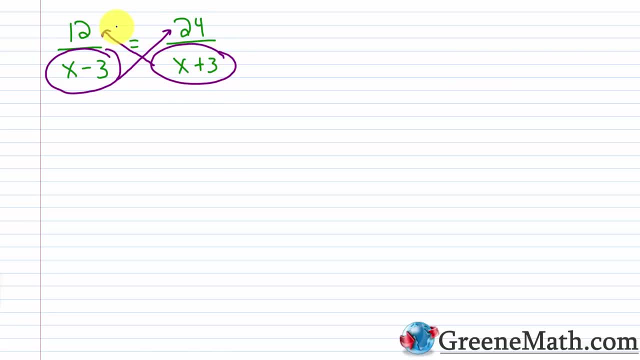 plus 3, that quantity times 12.. And why is that a shortcut? Well, the LCD here is going to be what It's: x minus 3 times x plus 3.. So if I multiply both sides of the equation by this LCD, well what's going to happen is this denominator here is going to cancel. 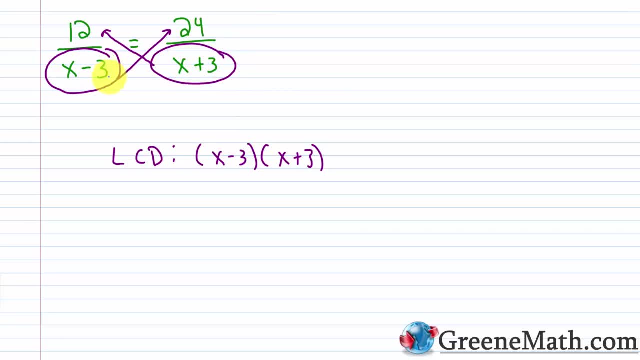 and I'm going to multiply 24 by x minus 3, which is exactly what I'm doing when I'm cross multiplying right. This would be 24 times. the quantity x minus 3 is equal to same thing over here. the x minus 3 would cancel and I'd be multiplying 12 by x plus 3.. That's what I'm. 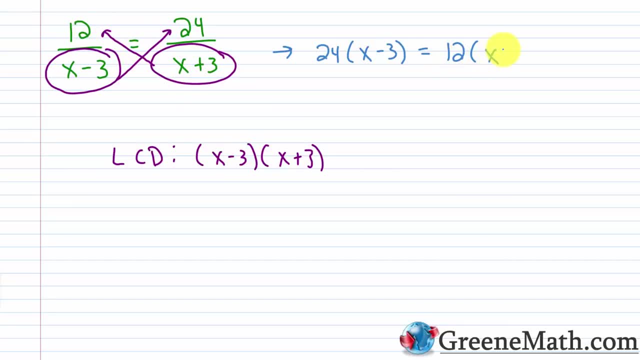 doing when I'm cross multiplying. So 12 times the quantity x plus 3.. So that's a little shortcut for you to kind of speed up the process if you get this scenario. So let's erase this real quick. And so 24 times x is 24x, and then 24 times negative 3 is going to give me. 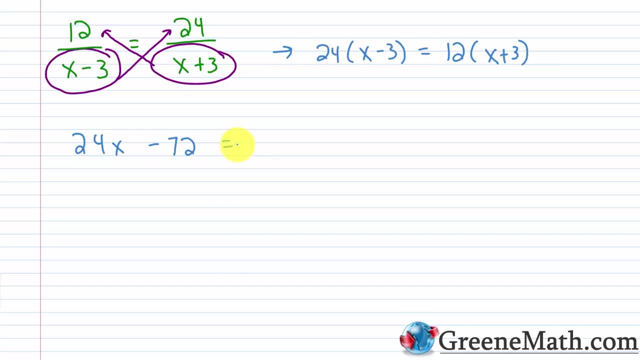 negative 72. And this is equal to over. here we have 12 times x, that's 12x. And then we have 12 times 3,, that's 36.. Okay, so let's solve this equation Very. 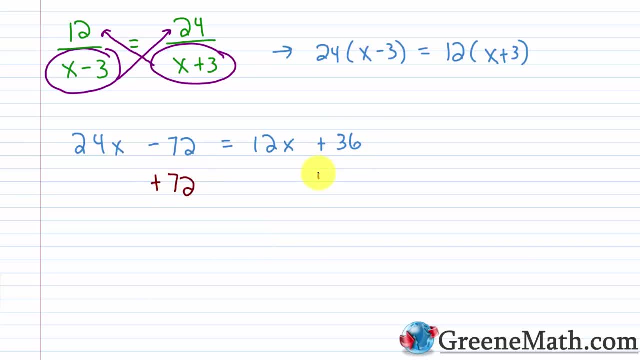 very easy to do. I'm just going to add 72 to both sides of the equation And I'm going to subtract 12x from both sides of the equation. So this is going to cancel and this is going to cancel. 24x minus 12x is 12x. 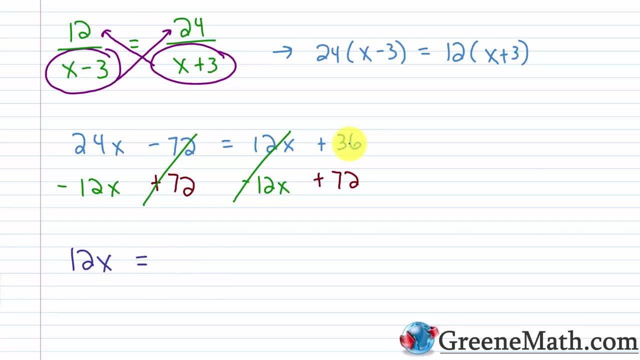 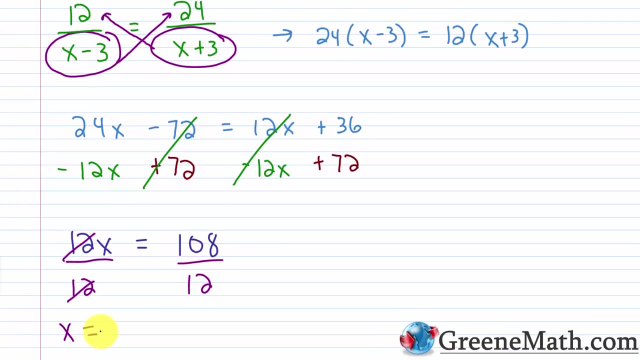 So this is 12x and this is equal to 36 plus 72,, which is 108.. Okay, as my last step here, I'm going to divide both sides of the equation by 12.. And this is going to cancel with this, and I'm going to have that x is equal to 9.. 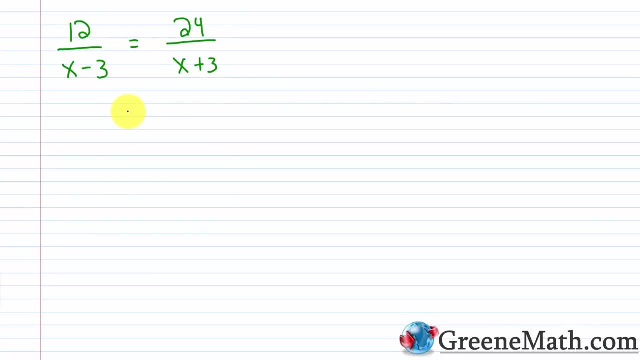 can do. this is we can find the LCD and multiply both sides of the equation by the LCD, clear the equation of any denominators and kind of go from there. But in this particular scenario the easiest thing to do would be to cross multiply. Remember that from proportions right, I can multiply x. 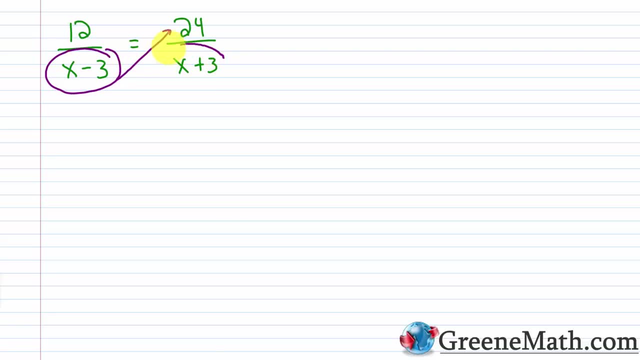 minus 3, that quantity times 24.. And I can multiply x plus 3, that quantity times 12.. And why is that a shortcut? Well, the LCD here is going to be what It's: x minus 3 times x plus 3.. So if I multiply both sides of the equation by this LCD, what's? 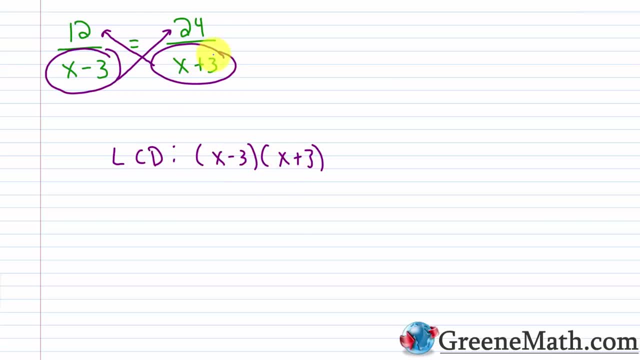 going to happen is this denominator here is going to cancel, and I'm going to multiply 24 by x minus 3, which is exactly what I'm doing when I'm cross multiplying right. This would be 24 times the quantity. x minus 3 is equal to 24 times x plus 3.. So I'm going to do that and I'm going to do the 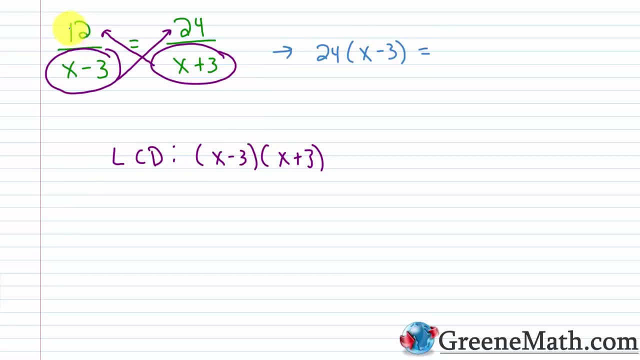 same thing here. I'm going to do the same thing here. I'm going to do the same thing here. I'm going to do the same thing over here. The x minus 3 would cancel, and I'd be multiplying 12 by x plus 3.. That's what. 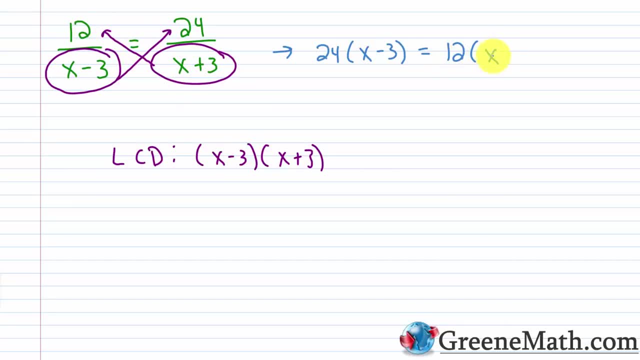 I'm doing when I'm cross multiplying. So 12 times the quantity x plus 3.. So that's a little shortcut for you to kind of speed up the process if you get this scenario. So let's erase this real quick. And so 24 times x is 24x, and then 24 times negative 3 is going to give me negative 72.. 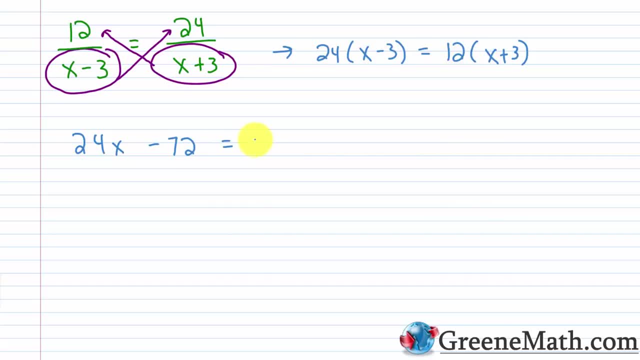 And this is equal to over. here we have 12 times x, that's 12x, and then we have 12 times 3,, that's 36.. Okay, so let's solve this equation. Very, very easy to do. I'm just going to add 72 to both sides of the equation. 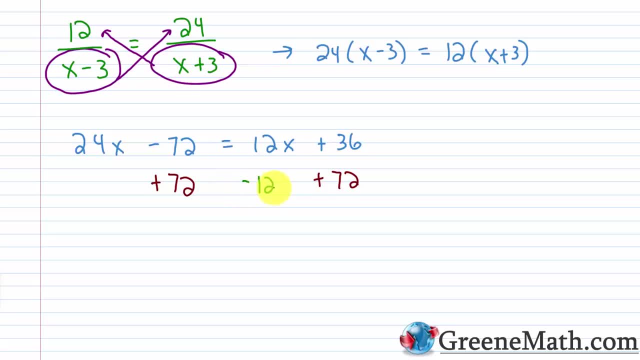 and I'm going to subtract 12x from both sides of the equation. So this is going to cancel and this is going to cancel. 24x minus 12x is 12x, So this is 12x and this is equal to 36 plus 72,. 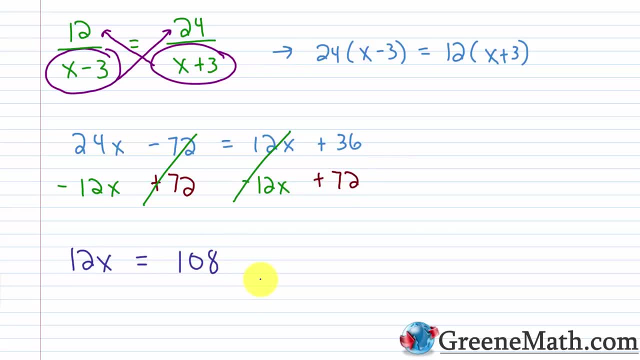 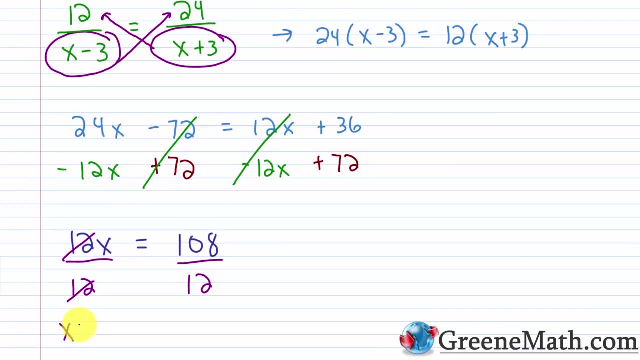 which is 108.. Okay, as my last step here, I'm going to divide both sides of the equation by 12, and this is going to cancel with this, and I'm going to have that x is equal to 9.. So I found the answer to the problem. x again was the speed of the boat in still water. 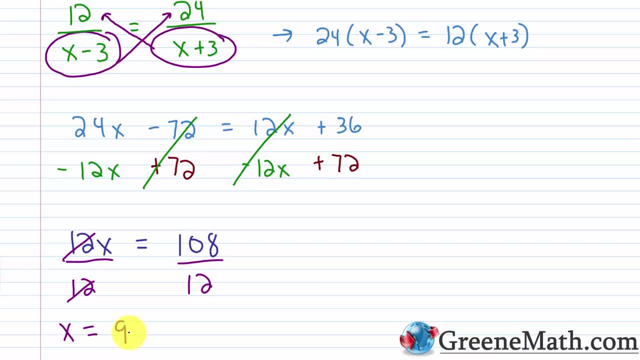 So I found the answer to the problem. x again was the speed of the boat in still water, and that's what I was trying to figure out. So x is equal to 9, so the speed of the boat in still water is equal to 9.. So I'm going to divide both sides of the equation by 12, and this is going to cancel with this and I'm going to have that x is equal to 9.. 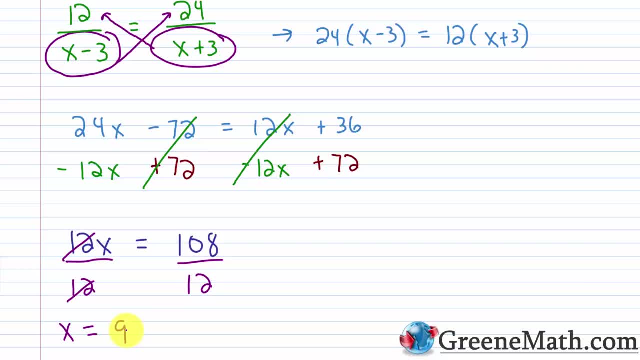 So I found the answer to the problem x is equal to 9, so the speed of the boat in still water is 9 miles per hour. So let's go back up to the top and write that. So I'm just going to write that the boat 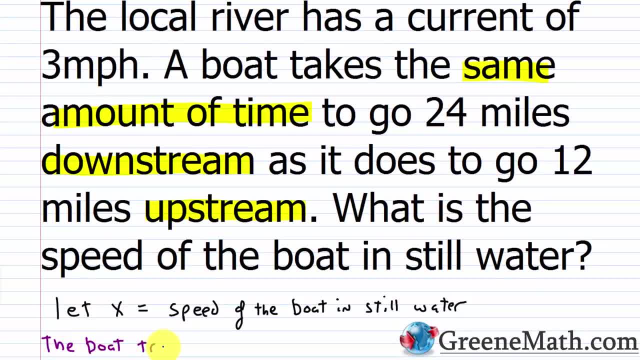 travels 9 miles per hour in still water, And that answers our question there. What is the speed of the boat in still water? So how would we check something like this? Well, let's read back through the problem real quick. So the local river has a current of 3 miles per hour. 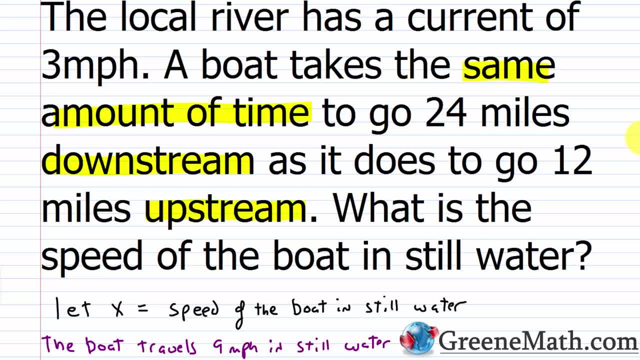 A boat takes the same amount of water as a boat. A boat takes the same amount of time to go 24 miles downstream again with the current as it does to go 12 miles upstream again against the current. So what is the speed of the boat in still water? 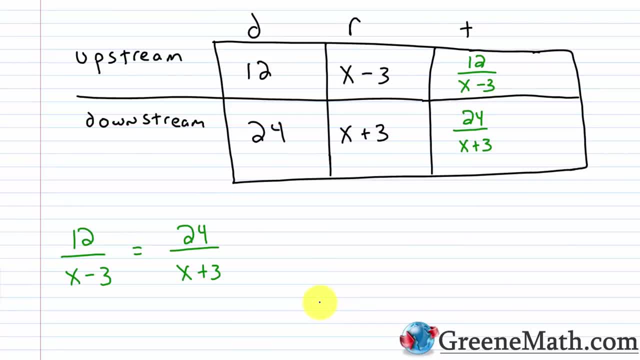 So I know at this point that upstream my rate of speed is going to be what? Well, x is 9.. So I plug in a 9 there. 9 minus 3 is 6.. So in other words, I know that the time that it takes to go 12 miles upstream, 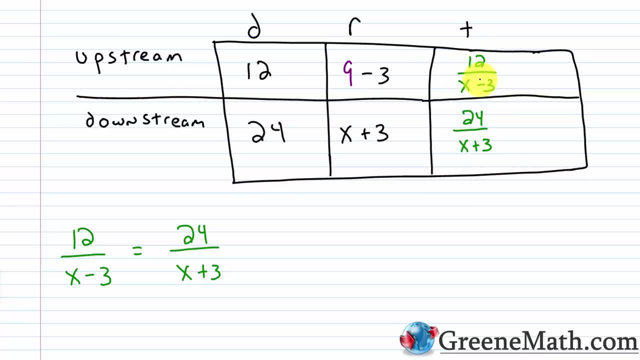 should be 12 over 9 minus 3.. Or 12 over 6,, which is 2.. And is that equal to the amount of time that it takes to go downstream? Well, my speed downstream if I replace this x with a 9,. 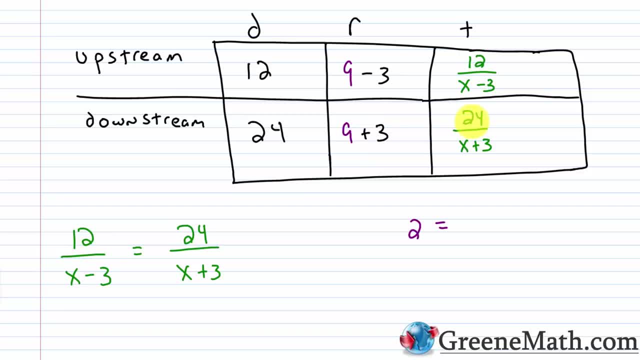 9 plus 3 is 12, is 12 miles an hour. You'd basically have 24 over again. 9 plus 3 is 12, so 24 over 12 would be 2.. So it takes the same amount of time, which is 2 hours. 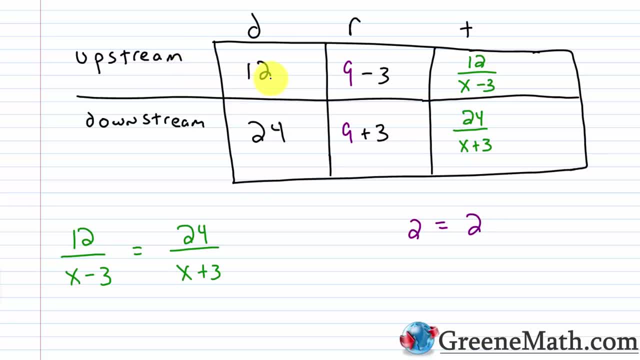 to go upstream 12 miles, as it does to go downstream 24 miles. So we have the correct answer here. Right, The speed of the boat in still water is 9 miles per hour. So the next type of problem we're going to deal with is known as a work rate problem. 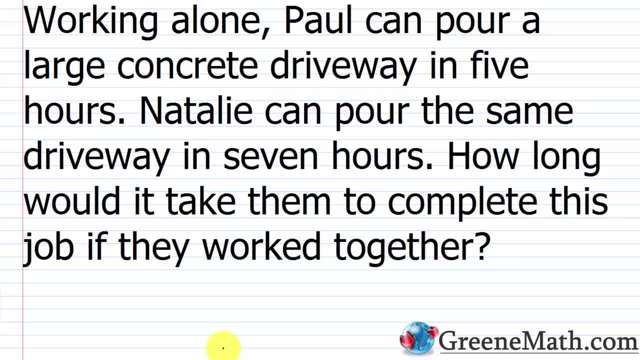 Or some of you will hear it called a rate of work problem. Either way, these type of problems involve how much time it takes to complete a job. So in this scenario, working alone, Paul can pour a large concrete driveway in 5 hours. 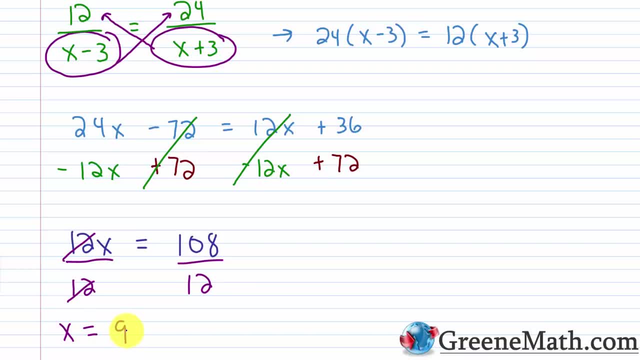 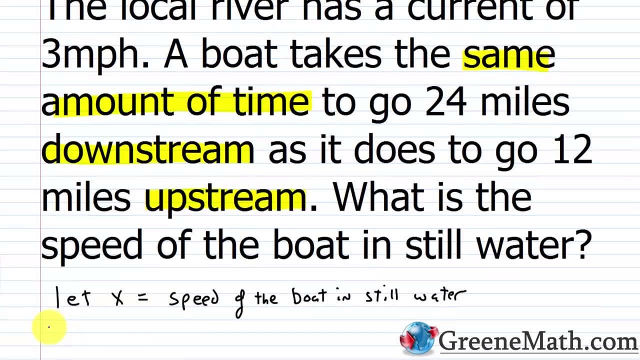 and that's what I was trying to figure out. So x is equal to 9, so the speed of the boat in still water is 9 miles per hour. So let's go back up to the top and write that. So I'm just going to write that the boat 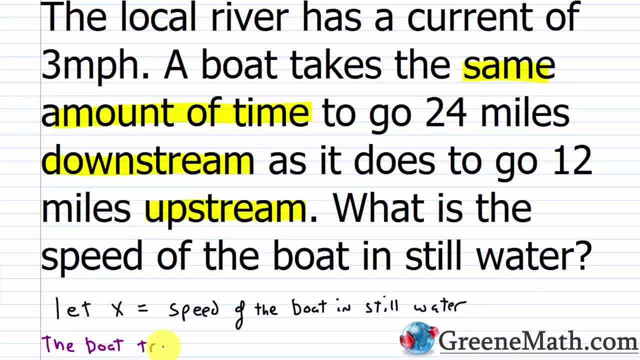 travels 9 miles per hour in still water, and that answers our question there. What is the speed of the boat in still water? So how would we check something like this? Well, let's read back through the problem real quick. So the local river has a current of 3 miles per hour. A boat takes the. same amount of time to go 24 miles downstream again with the current as it does to go 24 miles downstream. So the local river has a current of 3 miles per hour. A boat takes the same amount of time to go 24 miles downstream again with the current as it does to go 24 miles downstream. again with the current as it does to go 24 miles downstream. So the local river has a current of 3 miles per hour. So the local river has a current of 3 miles per hour. A boat takes the same amount of time to go 24 miles downstream. 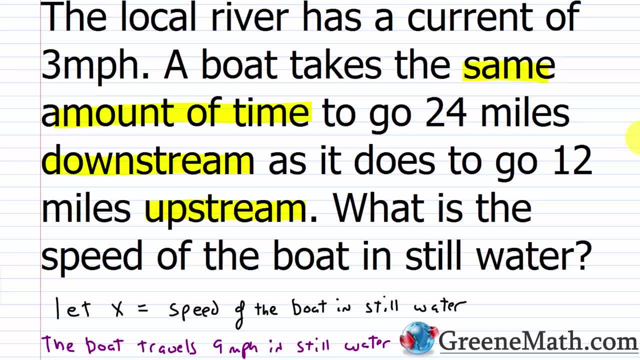 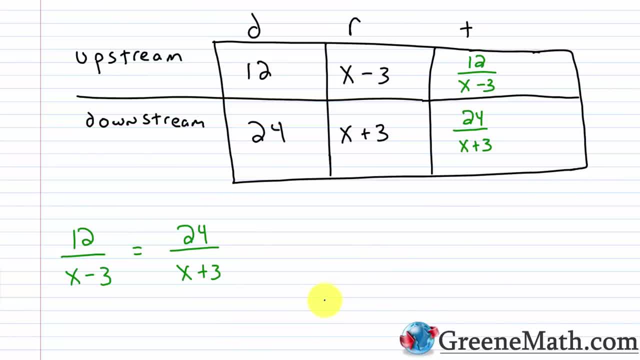 again with the current as it does, to go 24 miles upstream again against the current. So what is the speed of the boat in still water? So I know at this point that upstream my rate of speed is going to be what? Well, x is 9.. So I plug in a 9 there: 9 minus 3 is 6.. So in other words, I know. 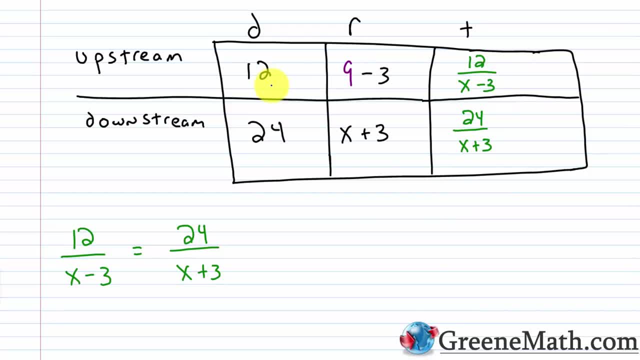 that the time that it takes to go 12 miles upstream should be 12 over 9 minus 3, or 12 over 6,, which is 2.. And is that equal to the amount of time that it takes to go downstream? Well, my speed downstream. 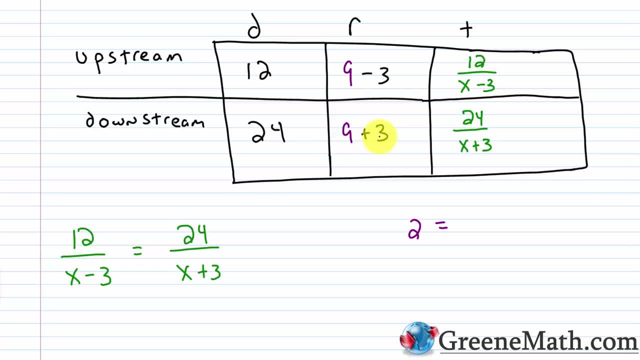 if I replace this x with a 9,- 9 plus 3 is 12, is 12 miles an hour- You'd basically have 24 over again, 9 plus 3 is 12,, so 24 over 12 would be 2.. So it takes the same amount of time. 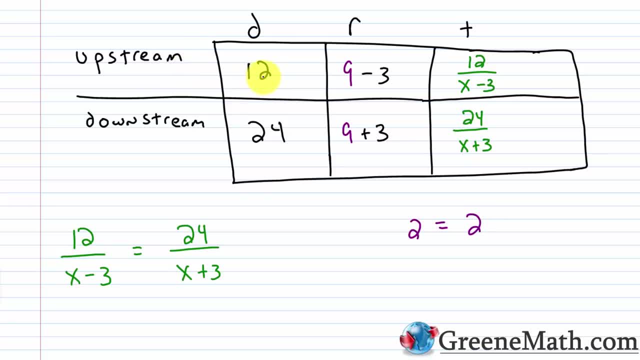 which is 2 hours to go upstream 12 miles, as it does to go downstream 24 miles. So we have the correct answer here. right, The speed of the boat is going to be 2 miles an hour. The speed of the boat in still water is 9 miles per hour. So the next type of problem: we're going. 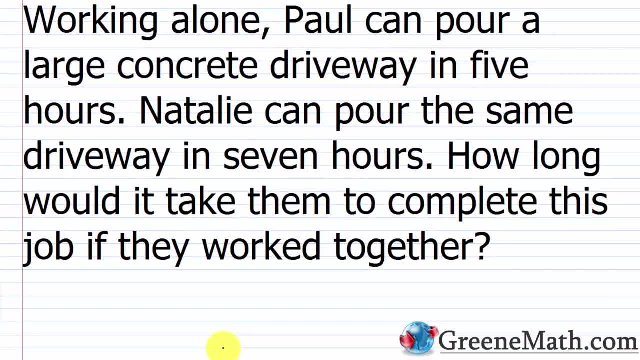 to deal with is known as a work rate problem, or some of you will hear it called a rate of work problem. Either way, these type of problems involve how much time it takes to complete a job. So in this scenario, working alone, Paul can pour a large concrete driveway in 5 hours. 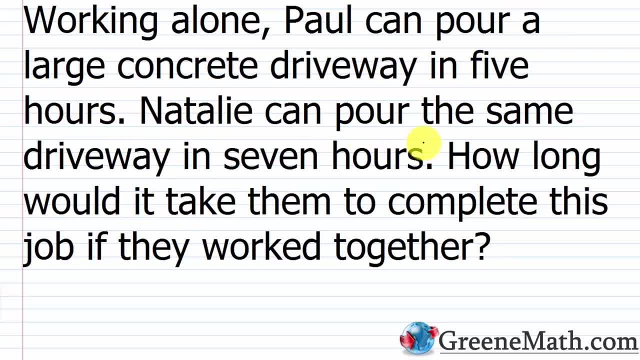 Natalie can pour the same driveway in 7 hours. How long would it take to complete this job if they worked together? So when you first start thinking about it, if you don't get any direction on it, it's kind of hard to figure out how to solve this. I know how long it would take for Paul. 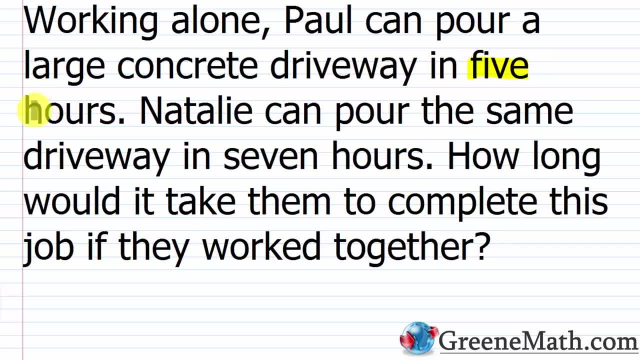 to pour a driveway: It's 5 hours. It says it right there. I know how long it would take for Natalie to pour the same driveway- It's 7 hours. But if I combine their work rates and they work together, how long is it going to take? 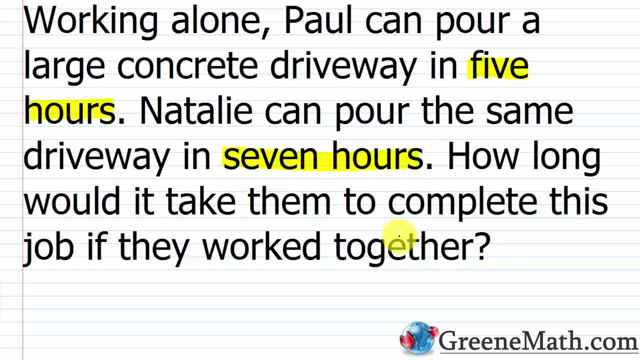 Well, the first thing I have to do is break this down into one unit of time. In this particular case, we're talking about hours. Now for these problems. you might talk about days or weeks or minutes, Whatever it is. 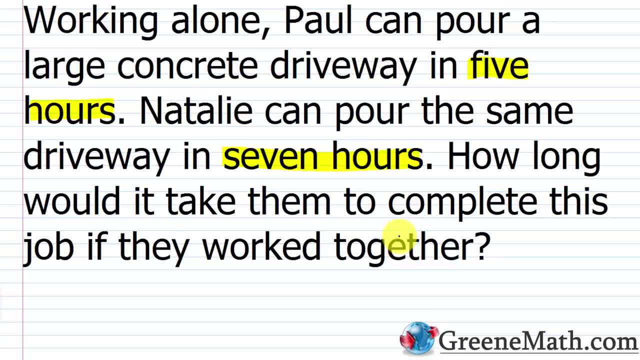 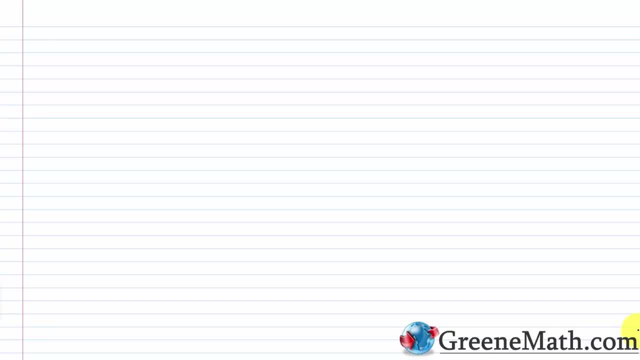 you're going to break it down into one of those units of time. So let me kind of scroll down a little bit, get some room going And I'm going to just think about: okay in one hour, because I want one unit of whatever time I'm dealing with. 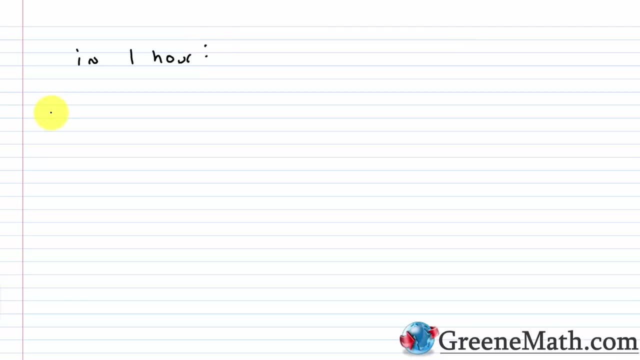 I'm dealing with hours, so I want one of those. What can Paul do in one hour? Well, Paul completes the job in five hours, So in one hour he's done one-fifth of the job, One-fifth of, you could say, the driveway, or of just the job, just to be generic. Then, Natalie, 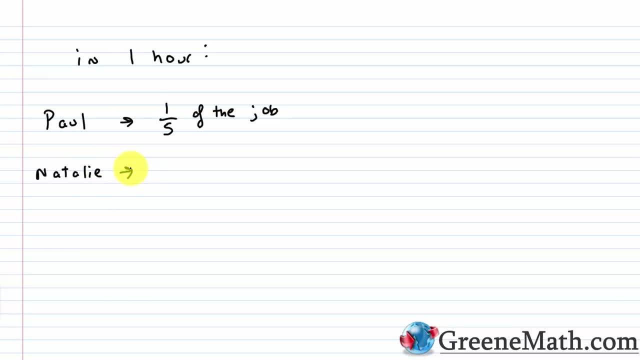 she's a little bit slower, She's a little bit slower, She's a little bit slower. It takes her seven hours to complete the job, So in one hour she's one-seventh complete, So one-seventh of the job. or again you could say: 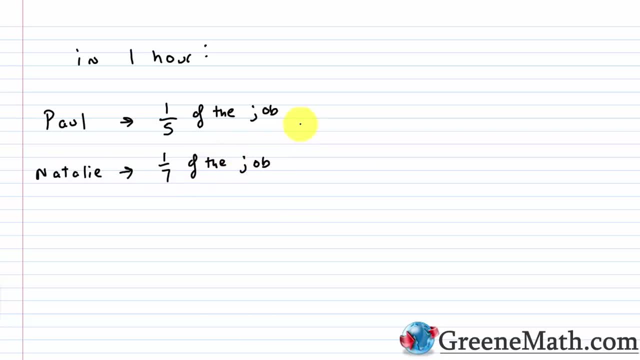 of the driveway. Okay, So what I want to do next is sum the individual contributions from these two people. If I do that, I'm going to get the amount of the job that is completed by both of them in a one-hour period, again working together. So what I want to do here is do one-fifth. That's the. 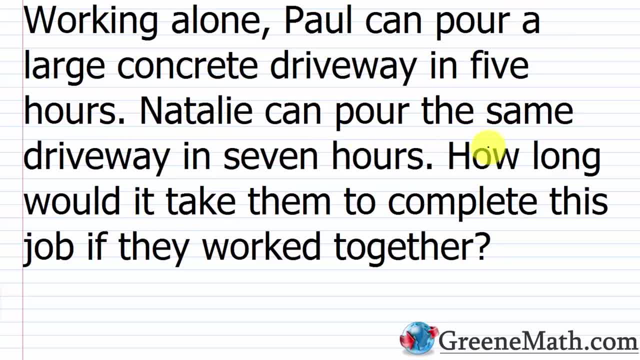 Natalie can pour the same driveway in 5 hours. Paul can pour the same driveway in 7 hours. How long would it take to complete this job if they worked together? So when you first start thinking about it, if you don't get any direction on it, 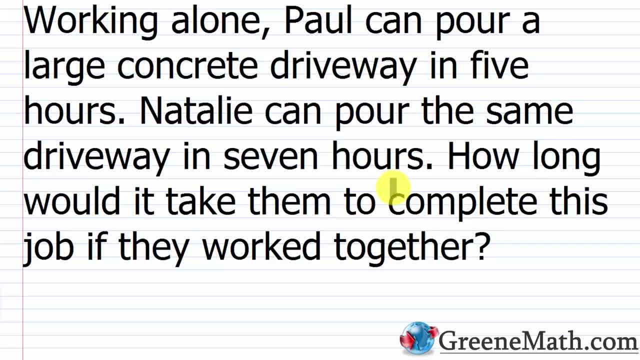 it's kind of hard to figure out how to solve this. I know how long it would take for Paul to pour a driveway. It's 5 hours, It says it right there. I know how long it would take for Natalie to pour the same driveway. 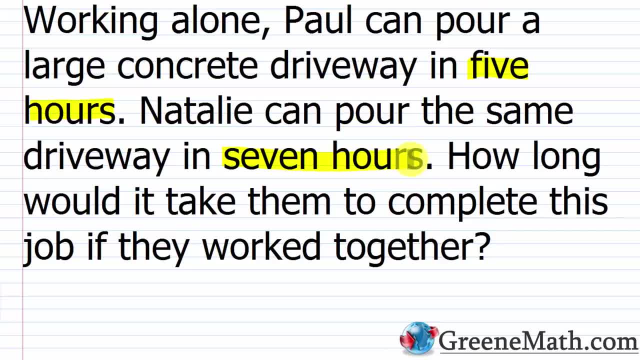 It's 7 hours, But if I combine their work rates and they work together, how long is it going to take? Well, the first thing I have to do is break this down into one unit of time. In this particular case, we're talking about hours. 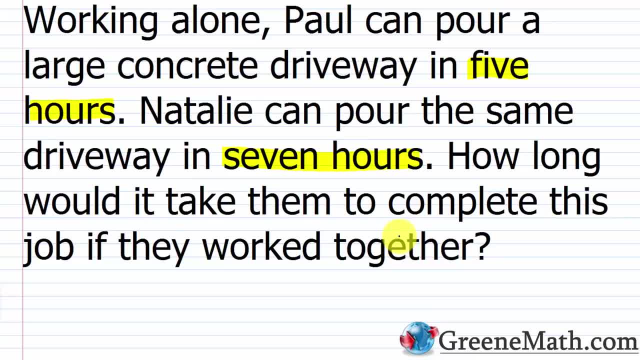 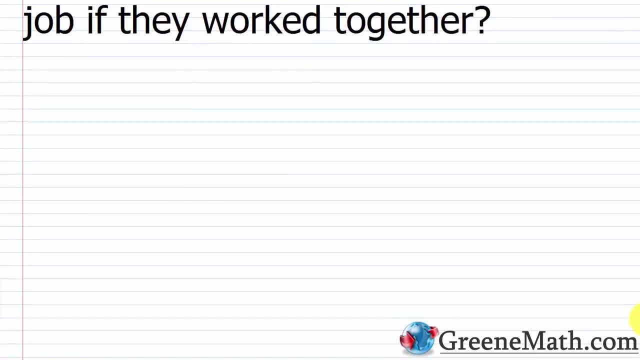 Now for these problems. you might talk about days or weeks or minutes, Whatever it is. you're going to break it down into one of those units of time, So let me kind of scroll down a little bit. get some room going. 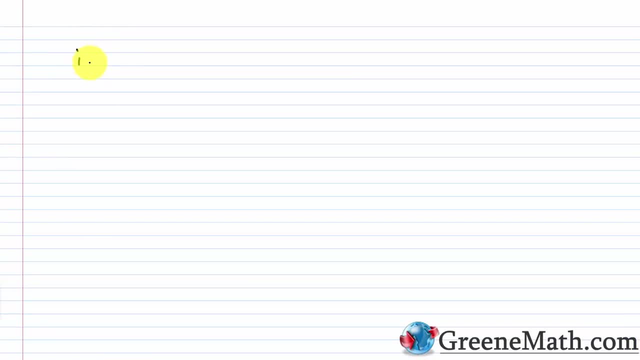 And I'm going to just think about: okay, in one hour, Because I want one unit of time. Okay, All right, So I want one unit of whatever time I'm dealing with. I'm dealing with hours, So I want one of those. 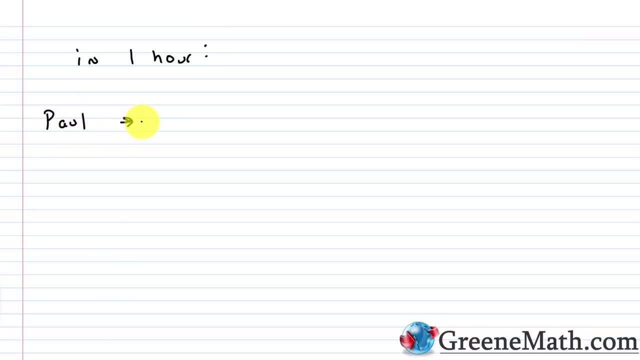 What can Paul do in one hour? Well, Paul completes the job in 5 hours. So in one hour he's done one-fifth of the job, One-fifth of, you could say, the driveway, or of just the job, just to be generic. 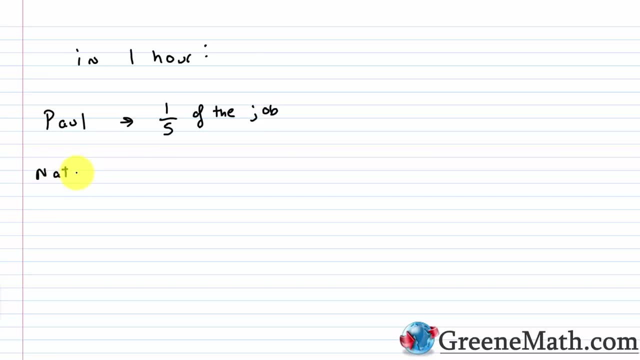 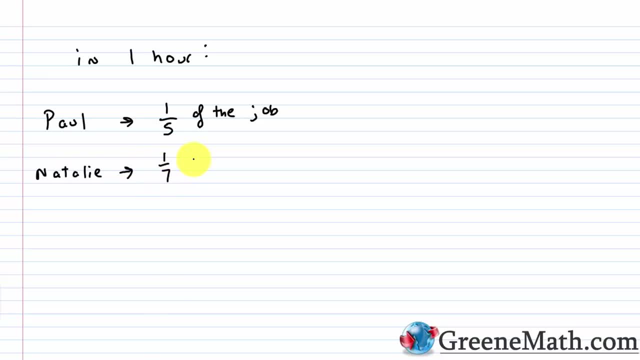 So in one hour she's one-seventh complete, So one-seventh of the job, or again you could say of the driveway. Okay, So what I want to do next is sum the individual contributions from these two people. If I do that, I'm going to get the amount of the job that is completed by both of them. 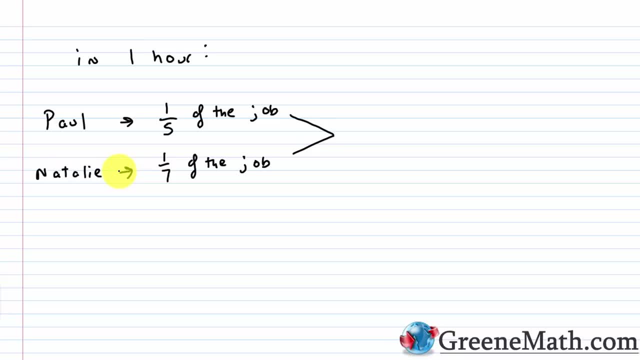 in a one-hour period, again working together. So what I want to do here is do one-fifth, That's the contribution from Paul, plus one-seventh, That's the contribution from Natalie, So I would get a common denominator here. 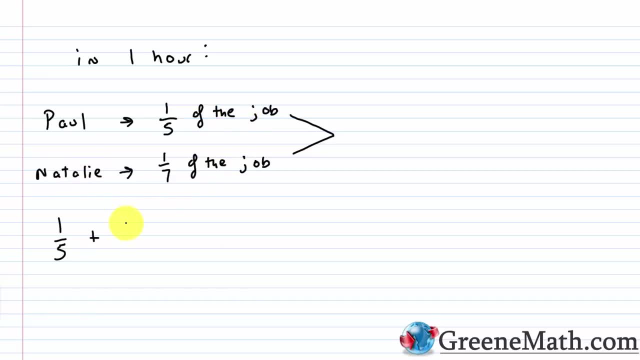 contribution from Paul. So I would get a common denominator here. This would be times five over five, This would be times seven over seven, And this would be what Seven plus five over seven times five is 35. So seven plus five is 12.. So this would be 12 over 35 here, And what 12 over 35 is, that's the contribution. 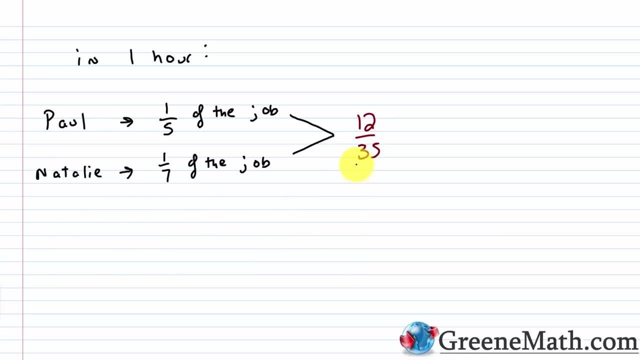 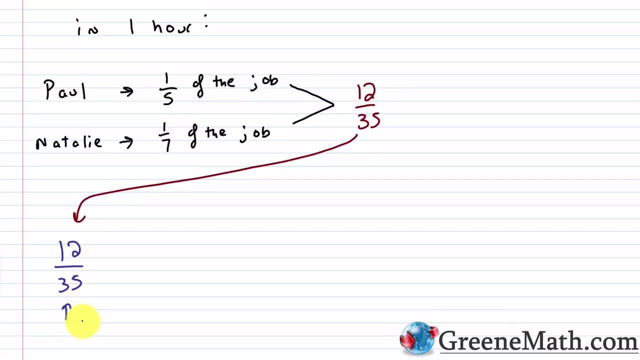 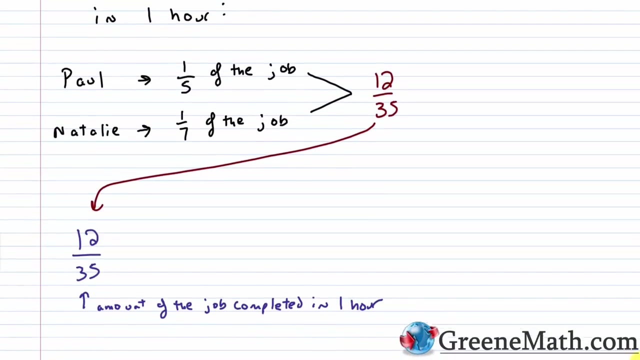 again by both of them in a one-hour period. So let me just kind of scroll this down here and just say 12: thirty-fifths is the amount of the job completed in one hour. Now the next thing I want to do, let me kind of go back up to the problem. 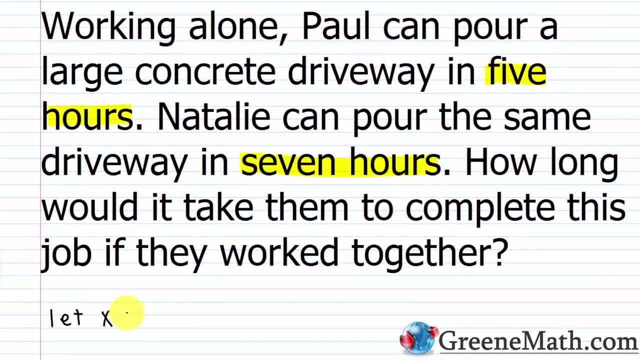 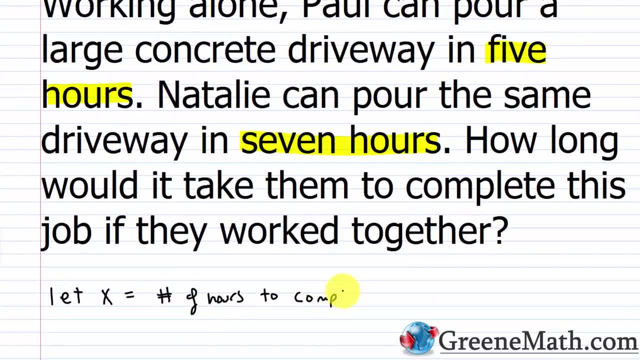 I'm going to let x here be equal to the number of hours to complete the job if they work together. So going back down, now we have 12 over 35 or 12. thirty-fifths is the amount of the job completed in one hour. 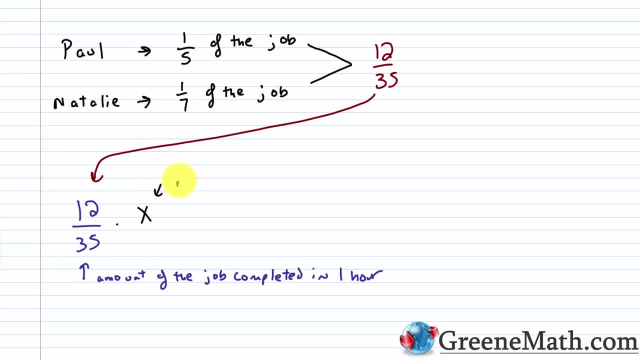 If I multiply this by x, which is the number of hours, the again number of hours to complete the job, I'm going to get one. Okay, and the reason we use one is it's one completed job. Now, to make this make sense for you, because I know when you start dealing with this it's like: why would you set it equal to one? so on and so forth. 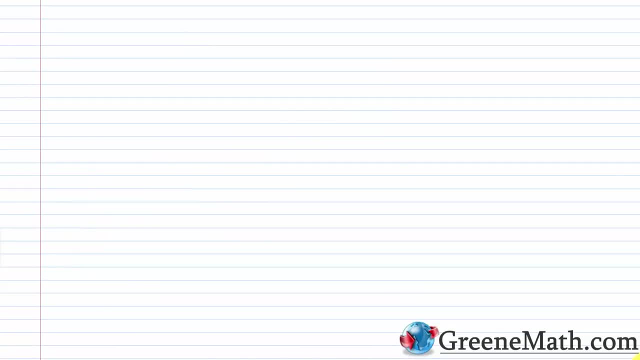 Let me just scroll down. I'm going to scroll down real quick and give you a very easy scenario. Let's say me and you paint a room in four hours working together. So that's very, very simple. So in one hour we would paint a fourth of the room. 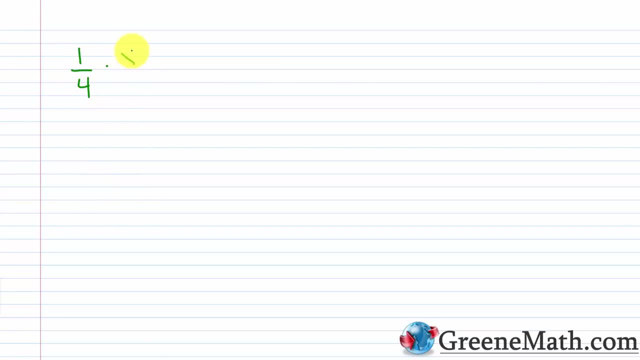 If I didn't know how many hours it would take. let's say I multiplied that by x and then I filled in that with a four. Well, I know that four times one-fourth is equal to one. It's because we're completing one room. 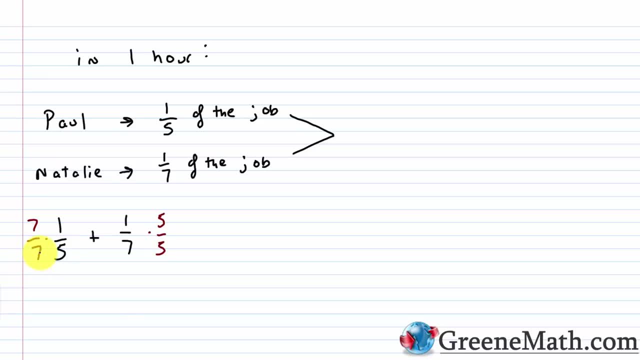 This would be times 5 over 5.. This would be times 7 over 7. And this would be what: 7 plus 5 over 7 times 5 is 35. So 7 plus 5 is 12.. 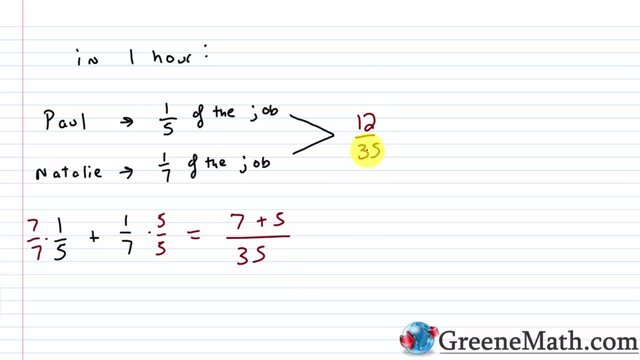 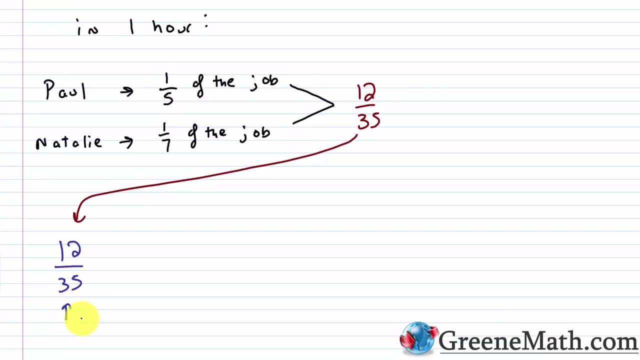 So this would be 12 over 35 here. And what 12 over 35 is, that's the contribution Again. So this would be both of them in a one-hour period. So let me just kind of scroll this down here and just say 12 thirty-fifths is the amount. 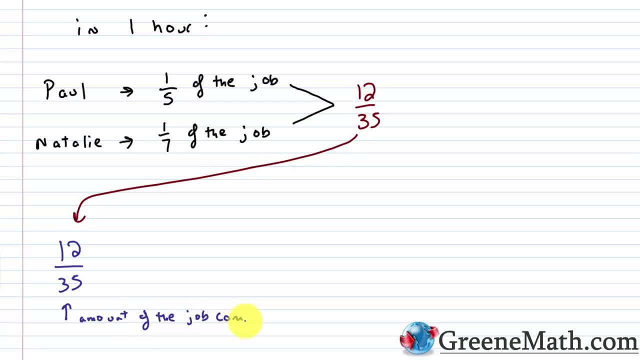 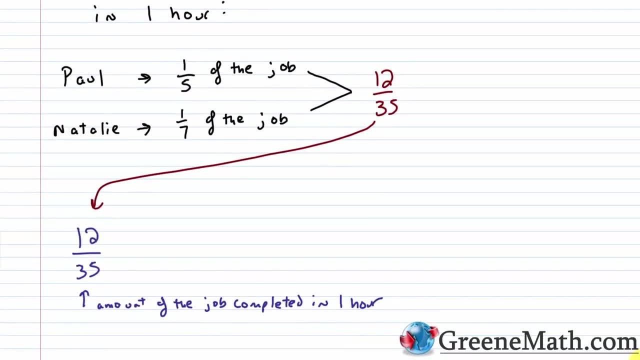 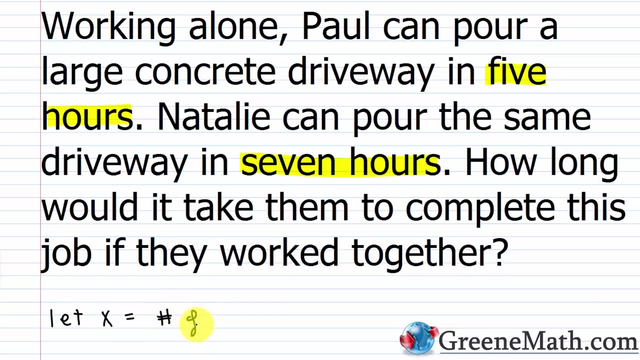 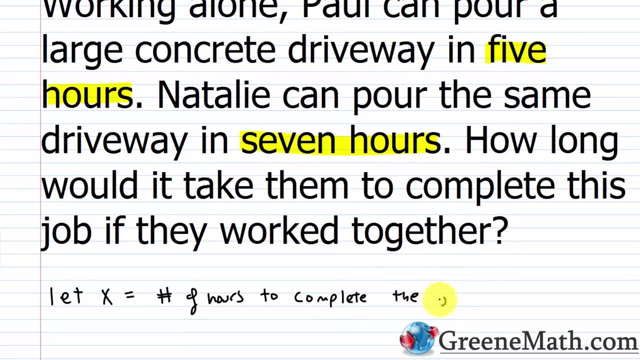 of the job completed in one hour. Now the next thing I want to do. let me kind of go back up to the problem. I'm going to let x here be equal to the number of hours to complete the job if they work together. 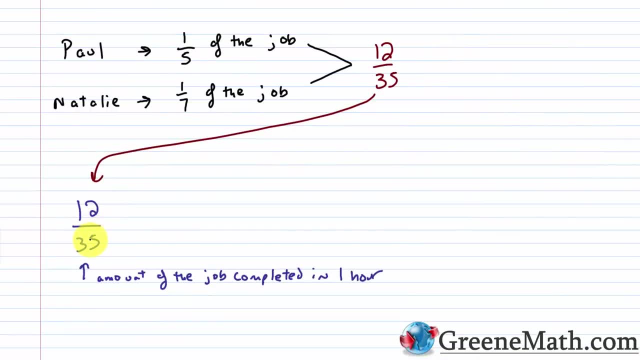 So, going back down now, we have 12 over 35, or 12. thirty-fifths is the amount of the job completed in one hour. If I multiply this by x, which is the number of hours The again. 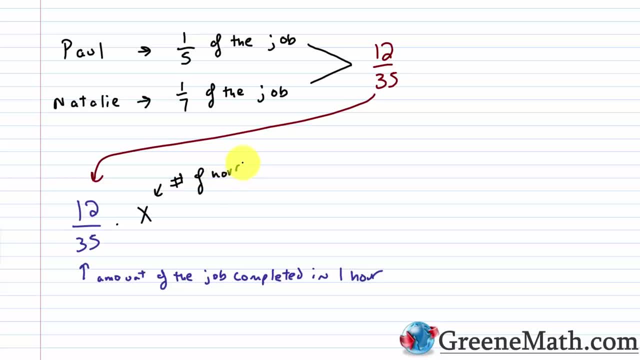 The number of hours to complete the job. I'm going to get 1.. Okay, And the reason we use 1 is it's one completed job. Now, to make this make sense for you, because I know when you start dealing with this it's. 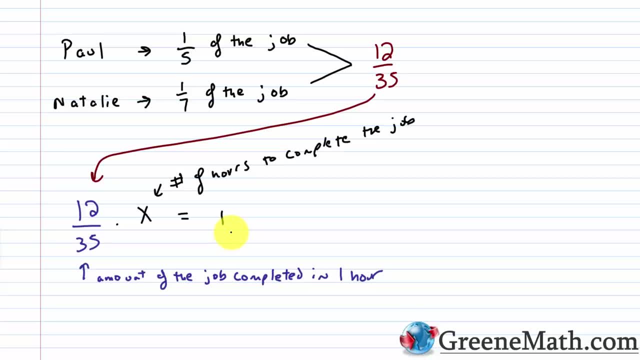 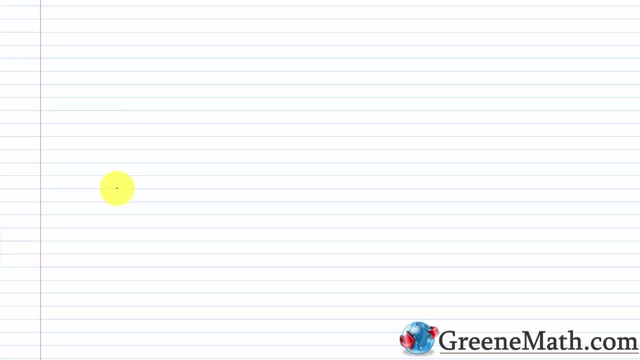 like: why would you set it equal to 1, so on and so forth. Let me just scroll down real quick and give you a very easy scenario. Let's say me and you paint a room. Let's say you paint a room In 4 hours working together. 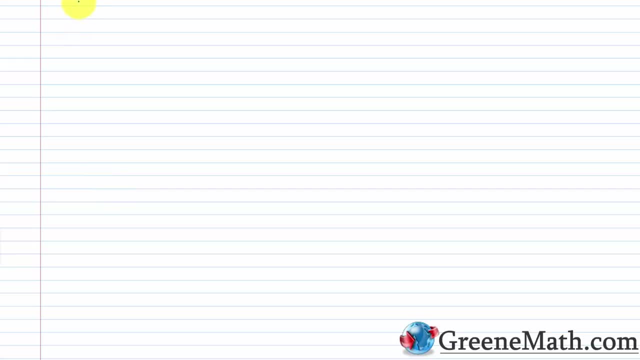 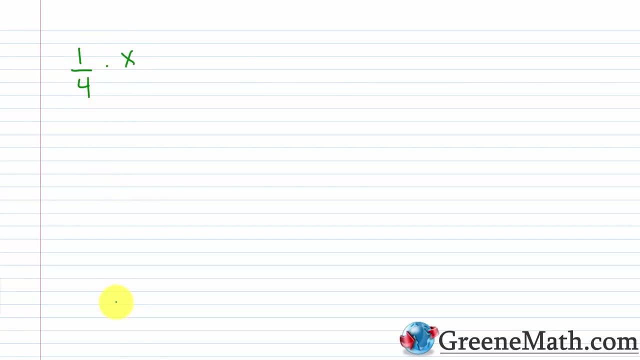 So that's very, very simple. So in one hour we would paint a fourth of the room. If I didn't know how many hours it would take, let's say I multiplied that by x and then I filled in that with a 4,. well, I know that 4 times 1, fourth is equal to 1.. 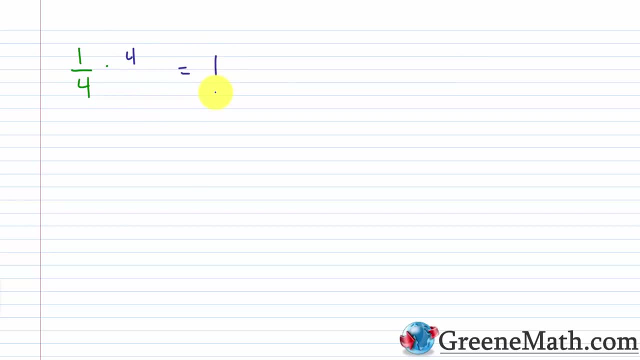 It's because we're completing one room or one job, however you want to think about that. So that's our goal. We're going to set this equal to 1, because we are trying to see how long it's going to take to complete one job. 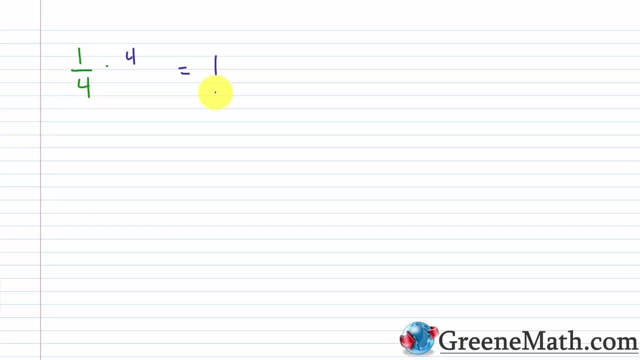 Or one job, However you want to think about that. So that's, our goal is to set this equal to one, because we are trying to see how long it's going to take to complete one job. Okay, so let's go back up. 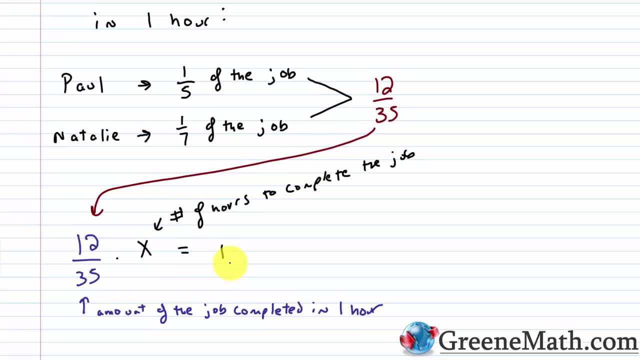 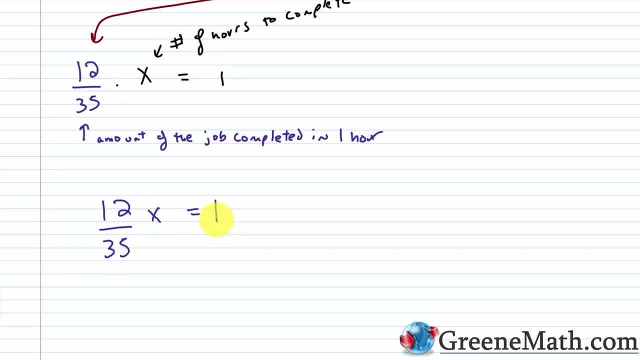 And now all we need to do is solve this very simple equation: If I have twelve thirty-fifths, x is equal to one. all I need to do is multiply both sides by the reciprocal. Multiply this by thirty-five twelfths. 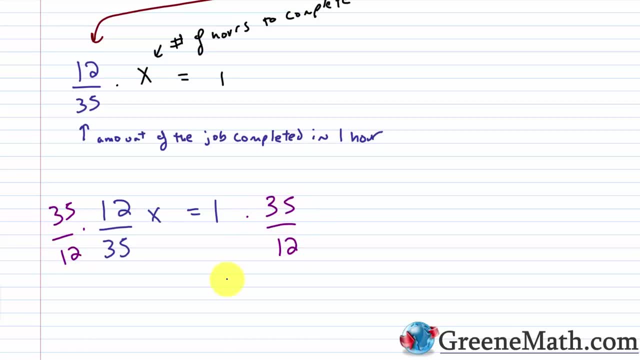 And this by thirty-fifths, And I'm going to get one. This is going to cancel And I'll have. x is equal to thirty-five twelfths. Now let's go back up to the top and make sense of this. 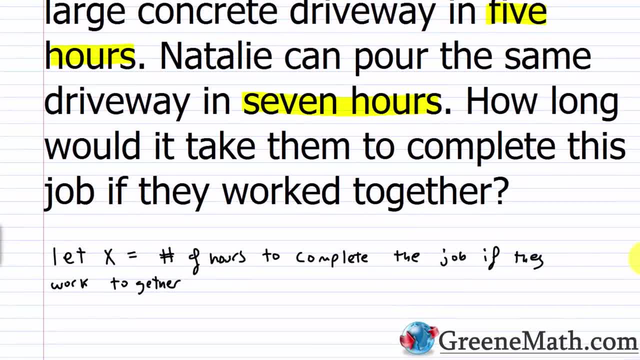 So I'm just going to answer it first. So how long would it take for them to complete this job? if they worked together, It would take Thirty-five, twelfths hours to complete the job, And you can do the division on that. 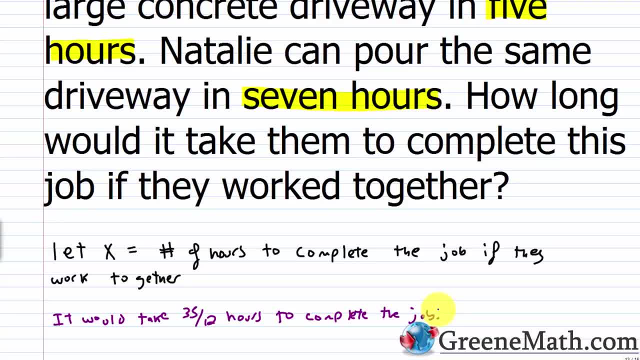 It's not going to give you an exact value, but it would be two point nine, one with a six. that repeats forever. So you could say about you know, approximately two point nine, two hours, if you wanted to just give an estimate. But if you wanted to be precise, which it's good to do on a test- I would just write that fraction that you got, which is thirty-five twelfths hours. 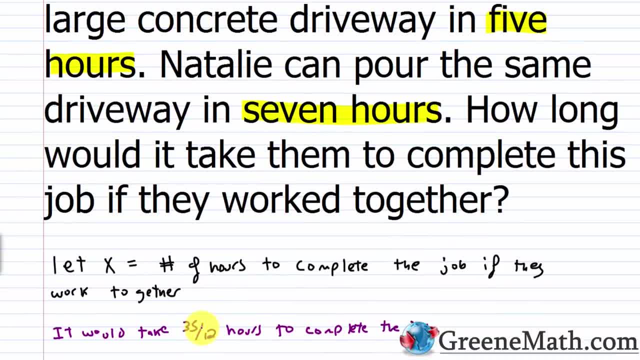 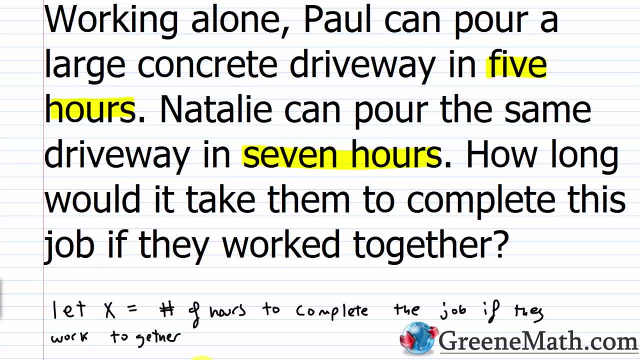 Now let's make sure that this makes sense. So again, working alone. Paul can pour a large concrete driveway in five hours. Natalie can pour the same driveway in seven hours. How long would it take for them to complete this job if they worked together? 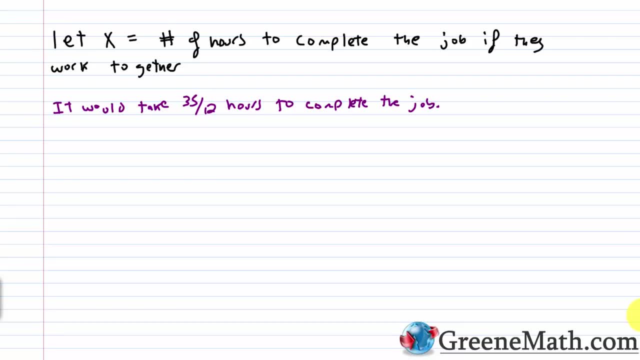 So what I'm going to do here is I'm going to take thirty-five, twelfths, Thirty-five, twelfths, which is the number of hours they work for. I'm going to multiply this by the rate of work, The rate of speed that Paul works at, which is one fifth. 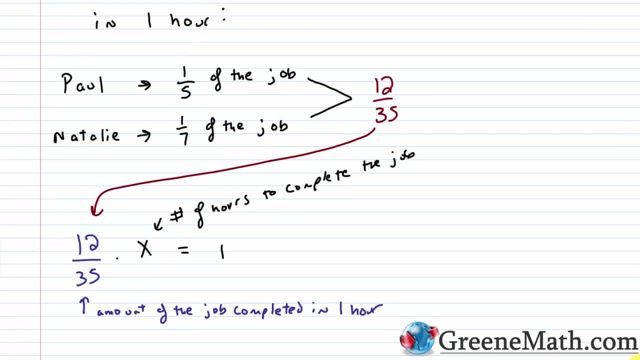 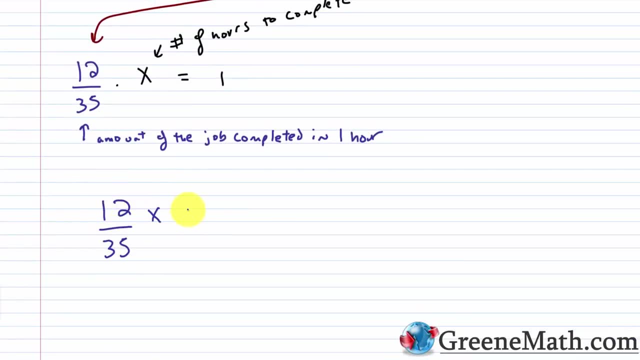 Okay, so let's go back up, And now. all we need to do is solve this very simple equation. If I have 12, thirty-fifths, x is equal to 1,. all I need to do is multiply both sides by the reciprocal. 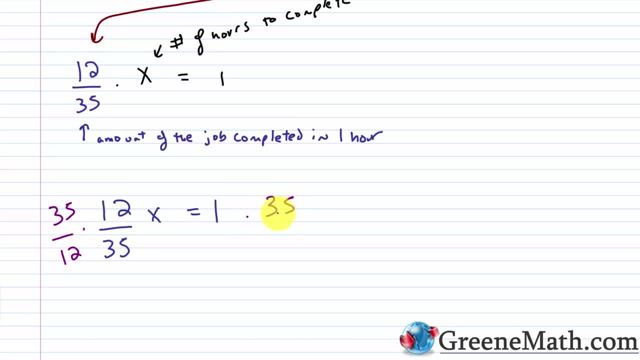 Multiply this by 35 twelfths and this by 35 twelfths and I'm going to get 1.. This is going to cancel. I'll have. x is equal to 30.. This is equal to 35 twelfths. 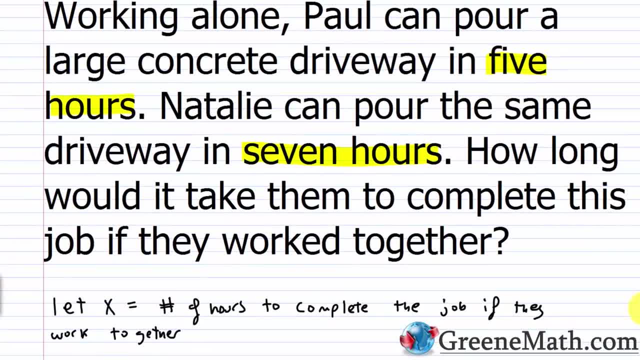 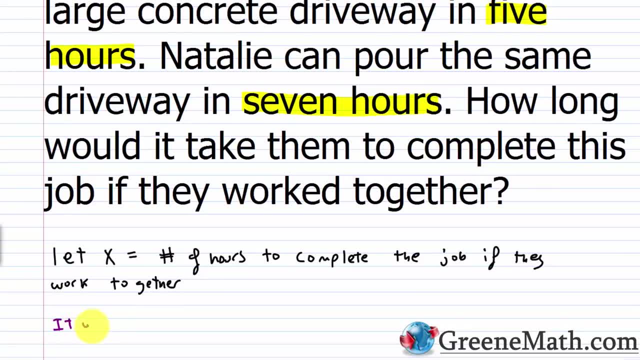 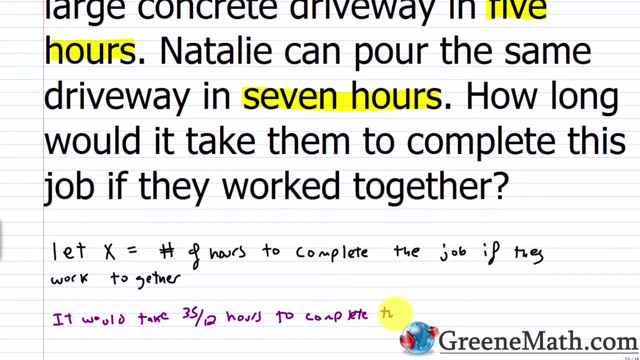 Now let's go back up to the top and make sense of this. So I'm just going to answer it first. So how long would it take for them to complete this job? if they worked together, It would take it would take 35 twelfths hours to complete the job. 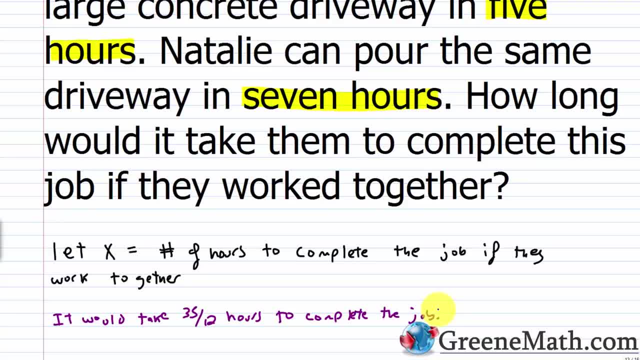 And you can do the division on this. It's not going to give you an exact value, but it would be 2.91 with a 6 that repeats forever. So you could say about you know, approximately 2.92 hours, if you wanted to just give an estimate. 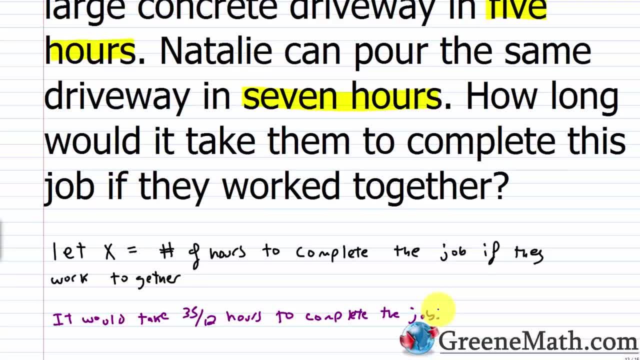 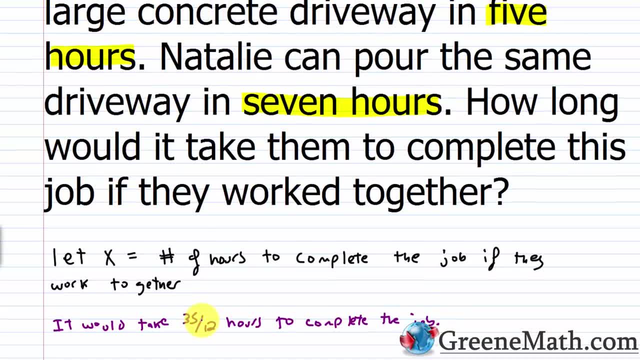 But if you wanted to be precise- which it's good to do on a test- I would just write that fraction that you got, which is 35 twelfths hours. Now, let's make sure that this makes sense. So again working alone. 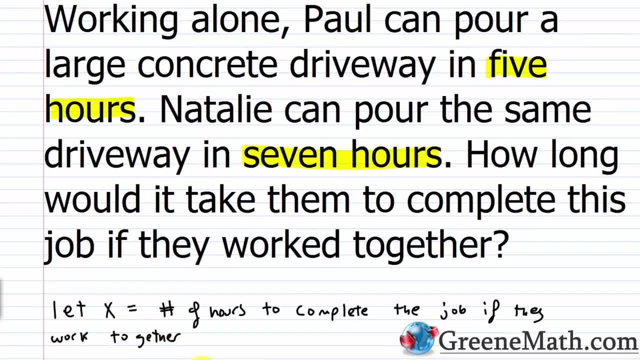 Paul can pour a lot of work into this, So I'm going to go ahead and do that. So I'm going to pour a large concrete driveway in five hours. Natalie can pour the same driveway in seven hours. How long would it take for them to complete this job if they worked together? 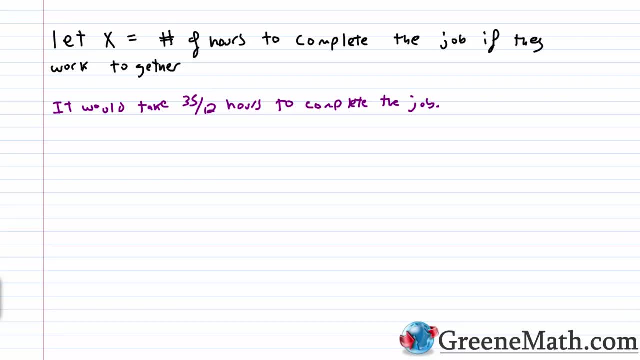 So what I'm going to do here is I'm going to take 35 twelfths. 35 twelfths, which is the number of hours they work for. I'm going to multiply this by the rate of speed that Paul works at, which is one fifth. 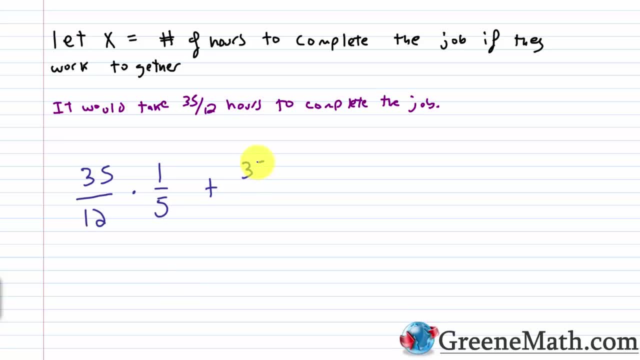 And then, plus I'm going to do 35 hours, 35 twelfths times the rate of speed that Natalie works at, which is one seventh, And let's see if this equals one right, One completed job. So this, divided by this, would give me seven.